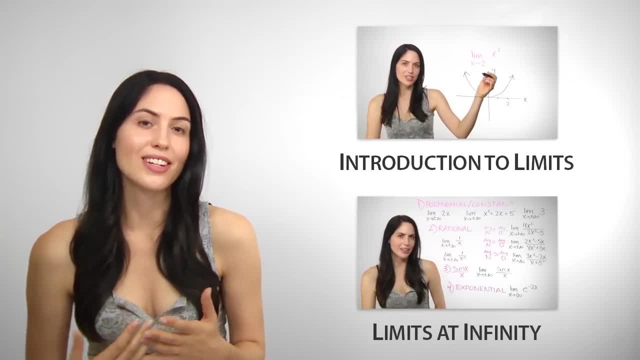 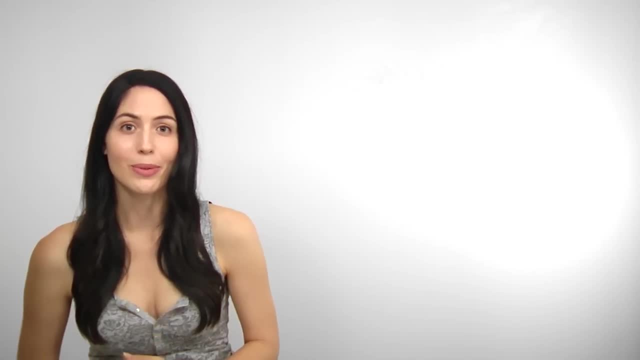 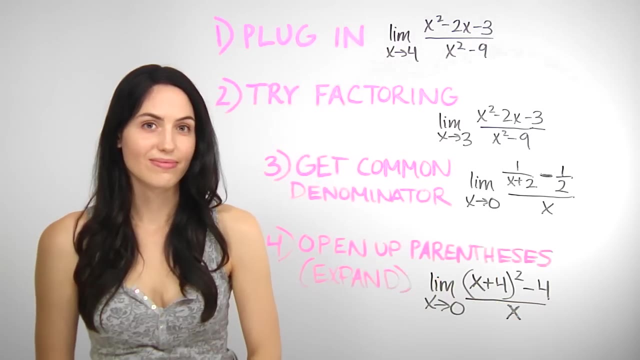 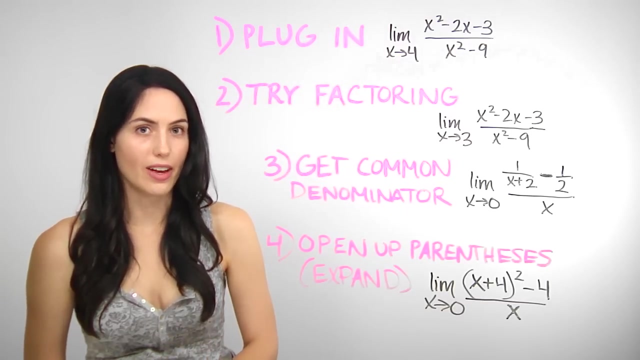 introduction video. If you're looking for how to find the limit at infinity, check out the limits at infinity video. But this is how to find the limit at a finite value, so let's look at the types I'm going to cover. Okay, these are the first four of seven ways to find the limit at a finite value. They 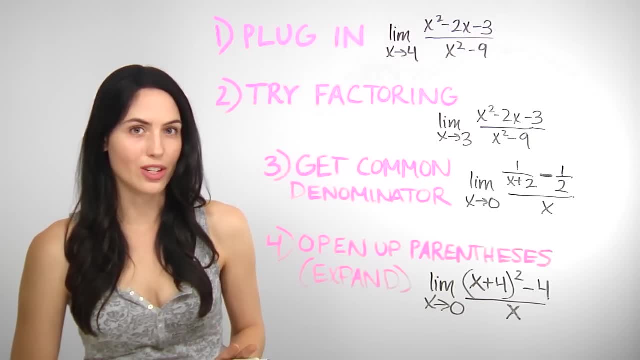 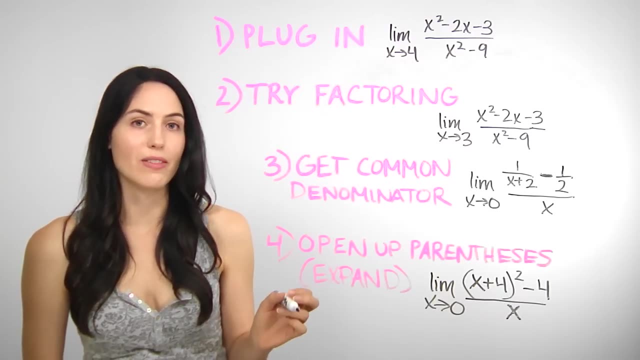 are the four main ways, most common strategies. If you already see the kind you're wondering about, the kind of problem you're working on, you can skip ahead. You can use the links in the video to skip directly to that part or you can check the links in the description. 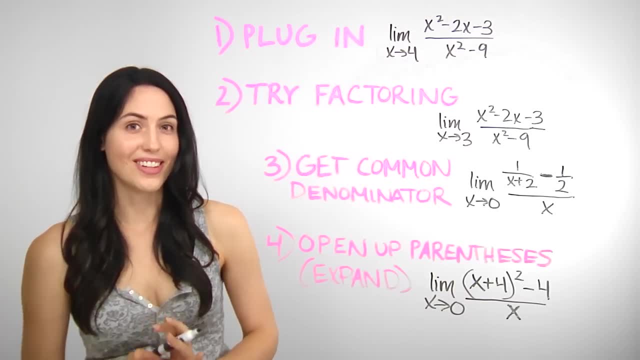 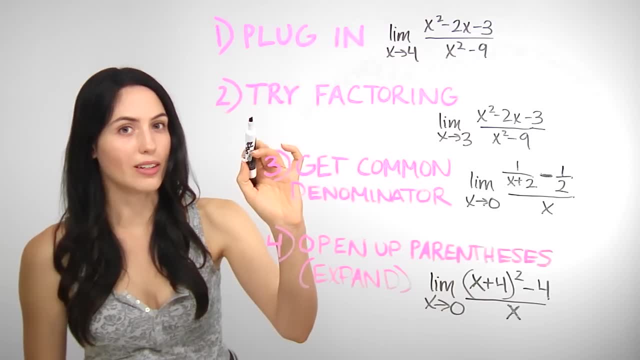 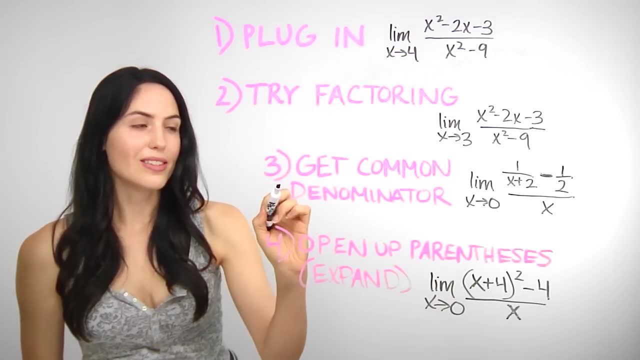 them. The first is to plug in if you can. If you can't- and I'll show you why- you might not be able to try factoring if possible. If not, see if you can get a common denominator. That means if you have something that looks like a fraction within a fraction. 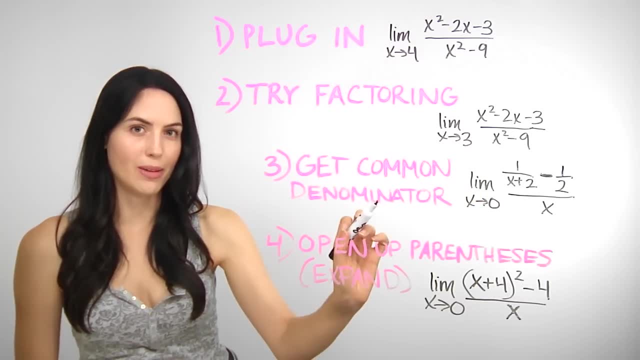 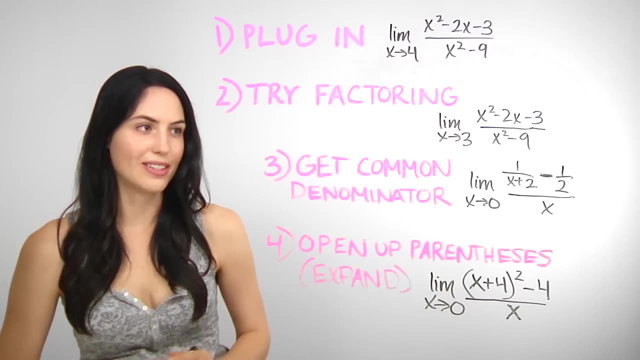 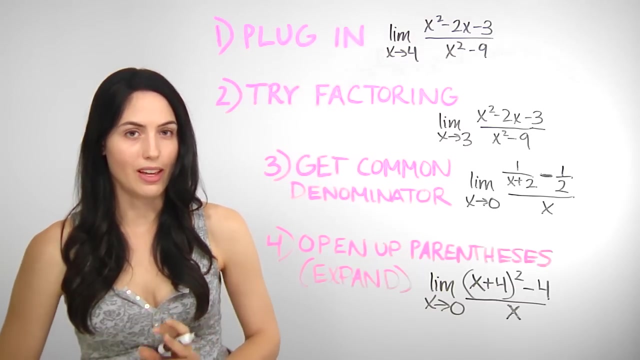 a complex rational expression, you might be able to get a common denominator. If not, see if you can expand, Open up parentheses, expand, simplify and then find the limit. These four cases cover most of the kind of limit problems at finite values. 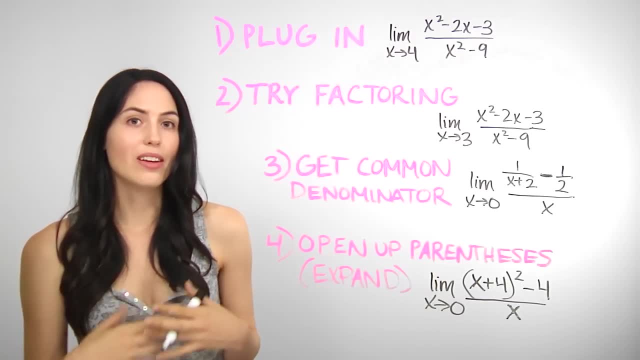 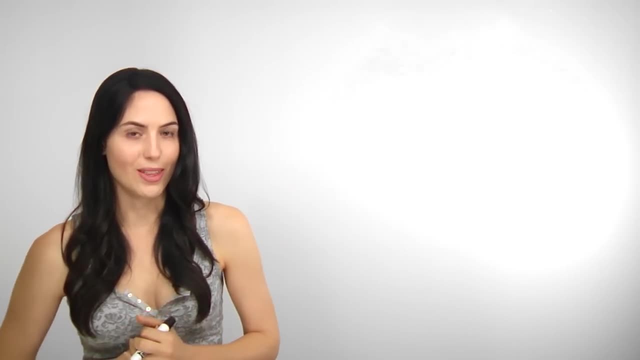 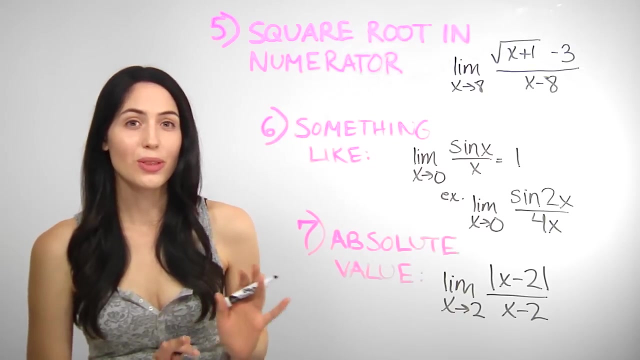 that you would get 90% of them, But there are a few oddball, miscellaneous misfit cases that come up, so let's look at those. Okay, these are the three miscellaneous oddball cases. If you're looking for one of these, I lied, They're not actually in this video. 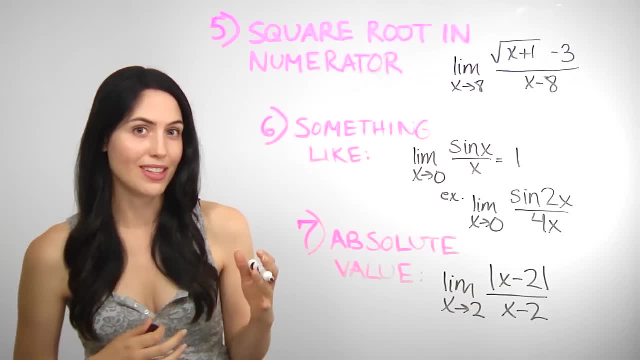 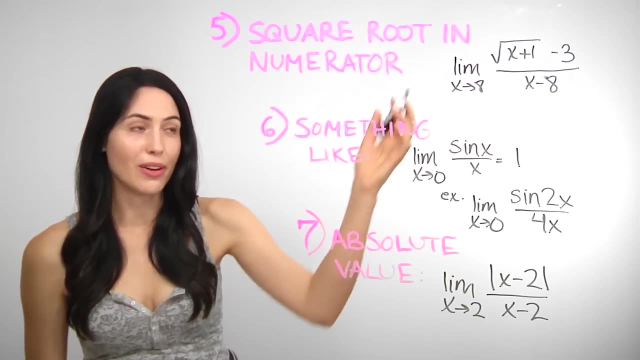 but you can use the links in this video to jump to that video where I explain these or look in the description for the video link. Basically, if you have a square root and a fraction in the numerator or something like sine x over x or absolute value, you'll need. 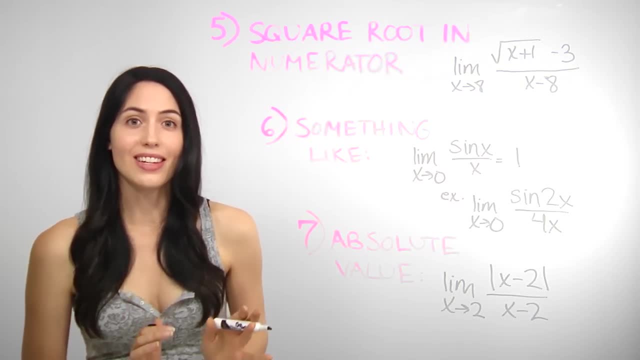 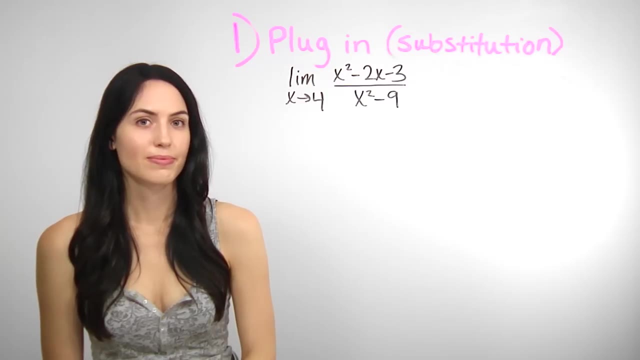 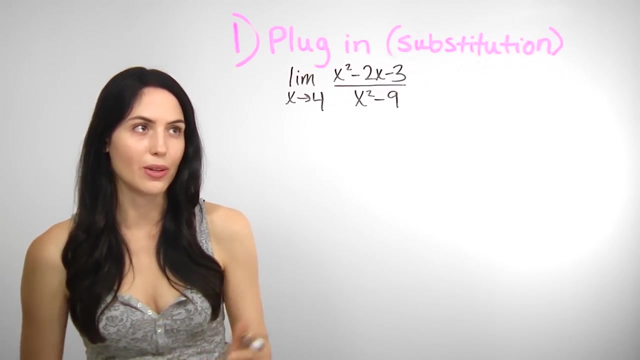 these strategies, But forget about those for now. Let's look at the four most common strategies. Okay, with these limit problems, the first thing you should always try is to plug in the value, Plug in 4 for x, everywhere x appears, and see if you get a value for the limit. 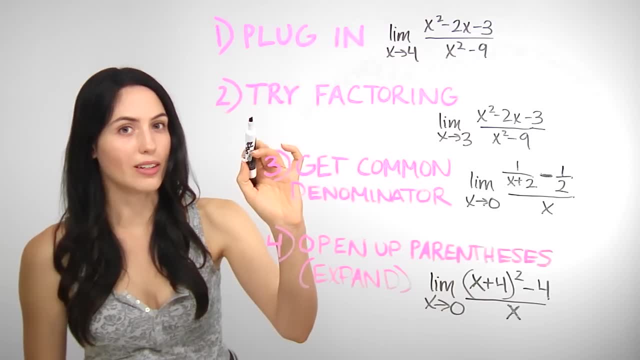 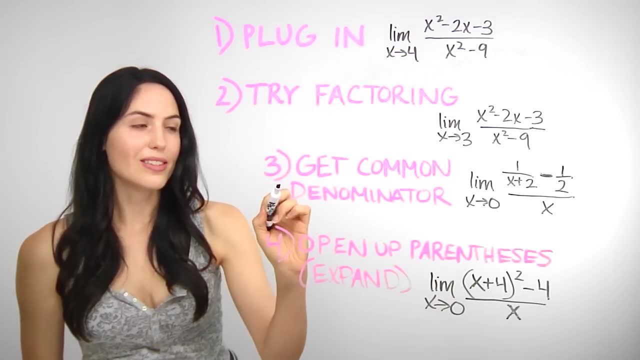 them. The first is to plug in if you can. If you can't- and I'll show you why- you might not be able to try factoring if possible. If not, see if you can get a common denominator. That means if you have something that looks like a fraction within a fraction. 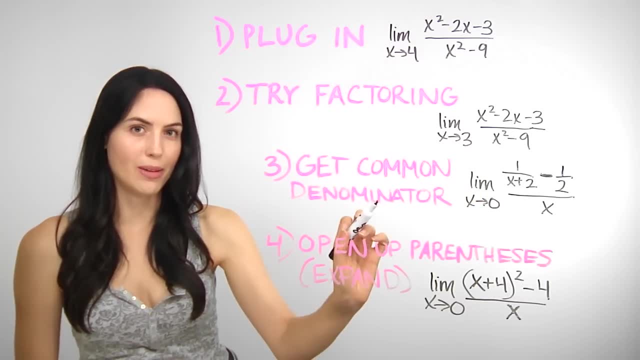 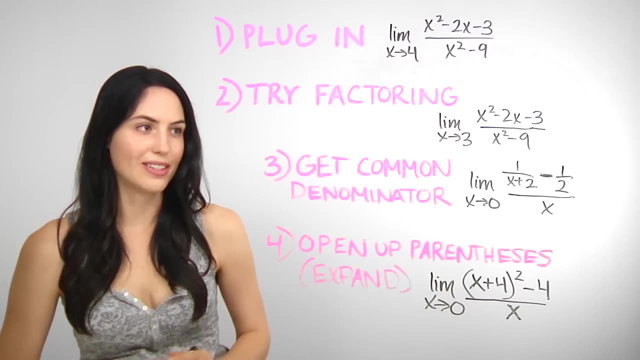 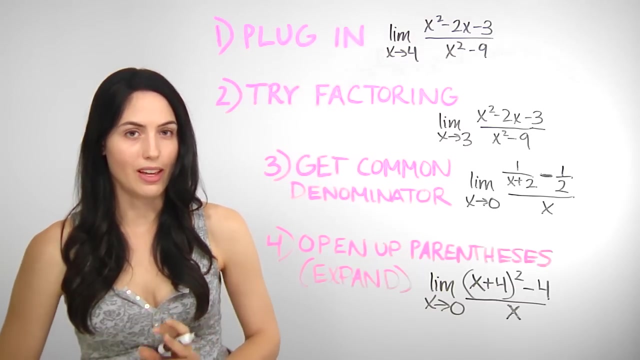 a complex rational expression, you might be able to get a common denominator. If not, see if you can expand, Open up parentheses, expand, simplify and then find the limit. These four cases cover most of the kind of limit problems at finite values. 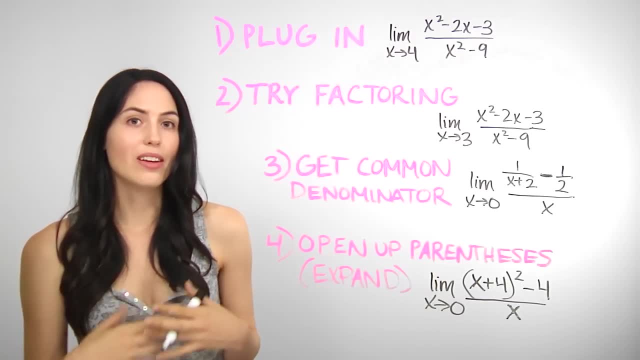 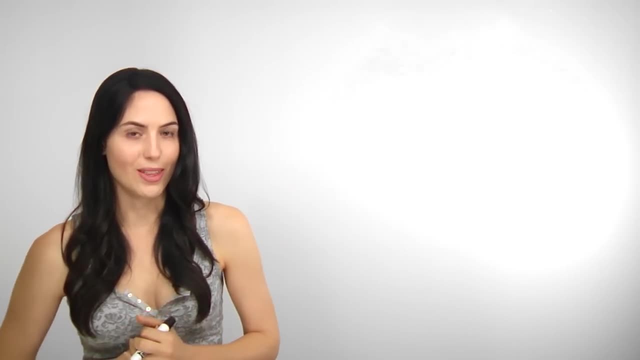 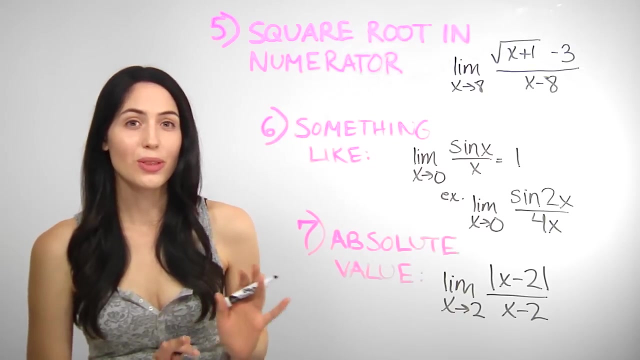 that you would get 90% of them, But there are a few oddball, miscellaneous misfit cases that come up, so let's look at those. Okay, these are the three miscellaneous oddball cases. If you're looking for one of these, I lied, They're not actually in this video. 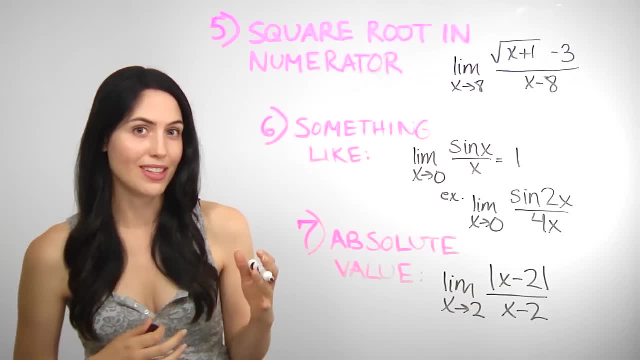 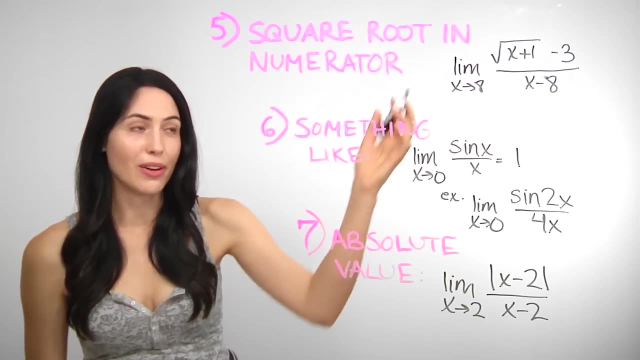 but you can use the links in this video to jump to that video where I explain these or look in the description for the video link. Basically, if you have a square root and a fraction in the numerator or something like sine x over x or absolute value, you'll need. 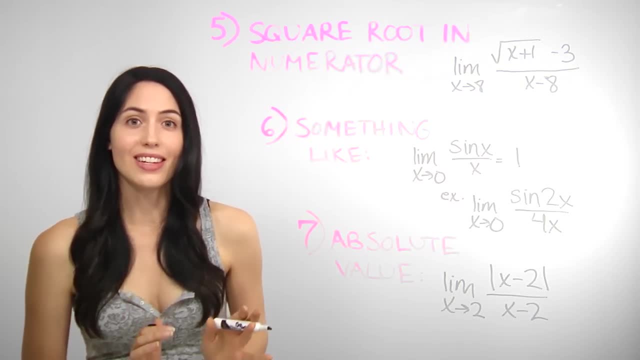 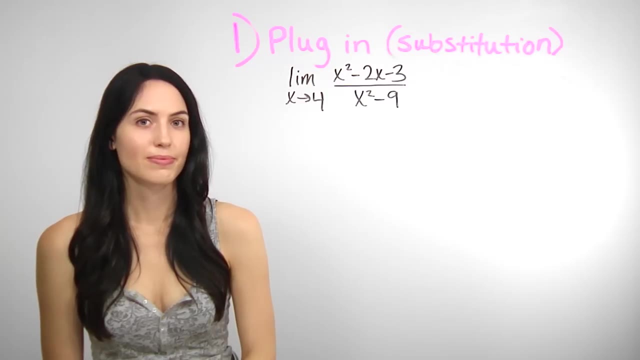 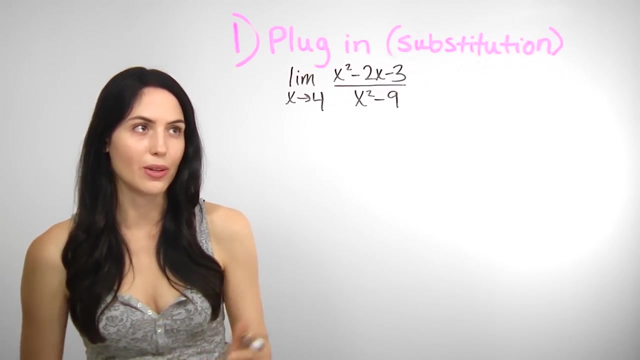 these strategies, But forget about those for now. Let's look at the four most common strategies. Okay, with these limit problems, the first thing you should always try is to plug in the value, Plug in 4 for x, everywhere x appears, and see if you get a value for the limit. 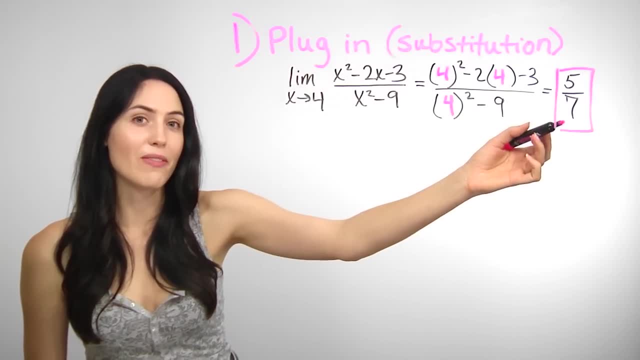 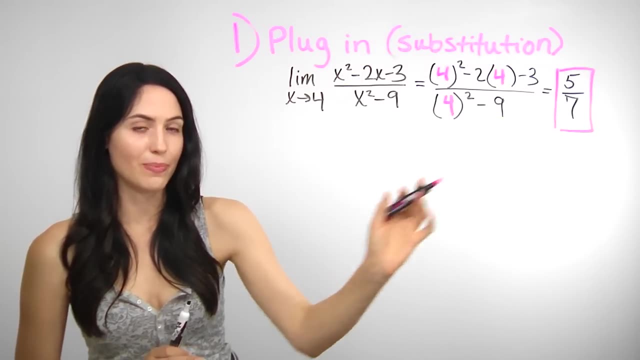 Okay, so you got an actual number for the limit, a finite value. 5- 7ths is a finite unique number. That is your limit. The limit is equal to 5- 7ths And you're done. But if you ever get a zero in the bottom in the denominator or the form, 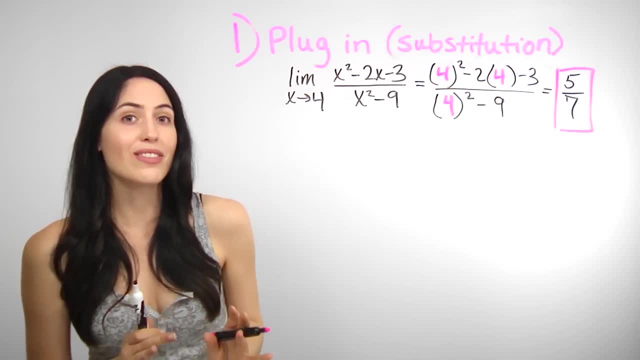 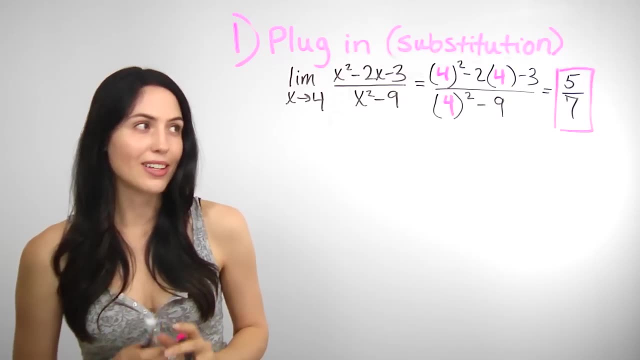 zero over zero, which is indeterminate. you have not found the limit. You're not done. You'll need another way, another technique. Before I show you another technique, here are some other common types of limits you can find just by plugging in. 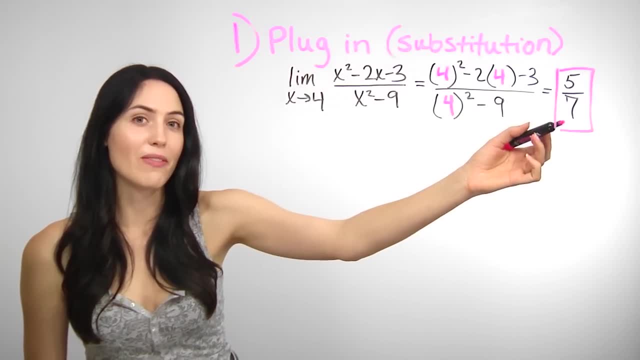 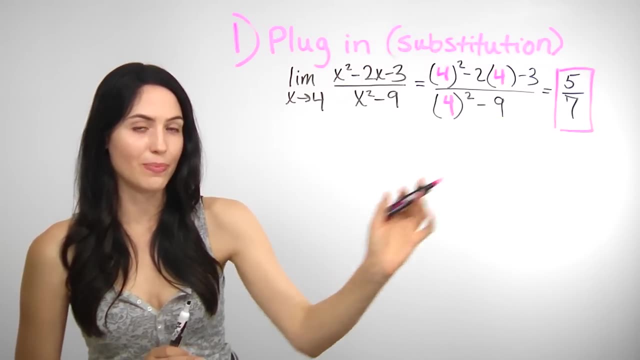 Okay, so you got an actual number for the limit, a finite value. 5- 7ths is a finite unique number. That is your limit. The limit is equal to 5- 7ths And you're done. But if you ever get a zero in the bottom in the denominator or the form 0 over 0,, 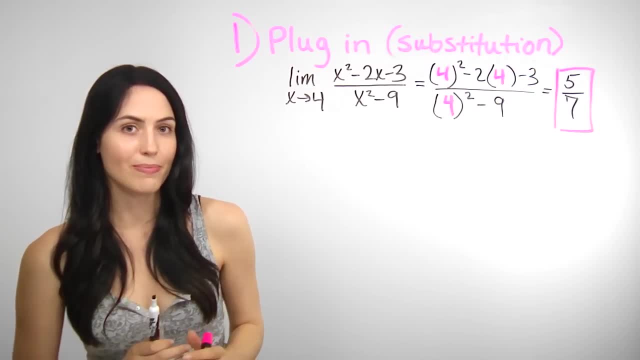 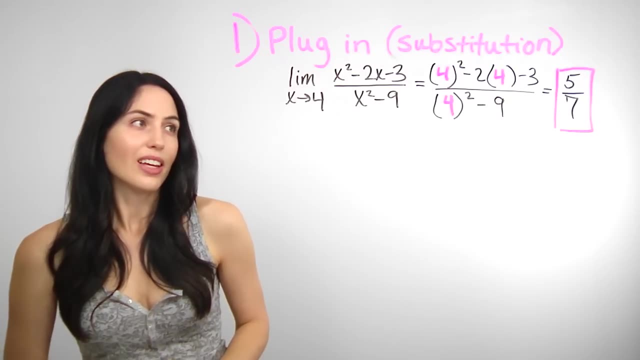 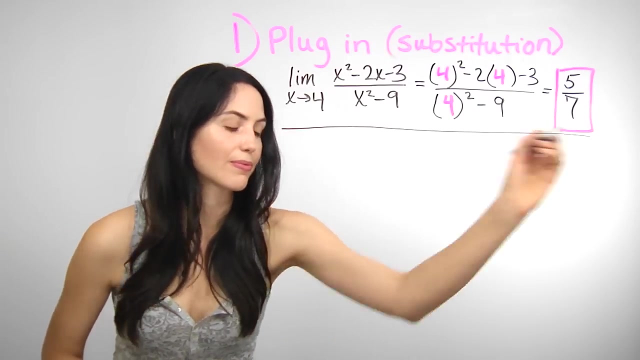 which is indeterminate. you have not found the limit, You're not done. You'll need another way, another technique. Before I show you another technique, here are some other common types of limits you can find just by plugging in. These are all other limits you can find just by plugging in. 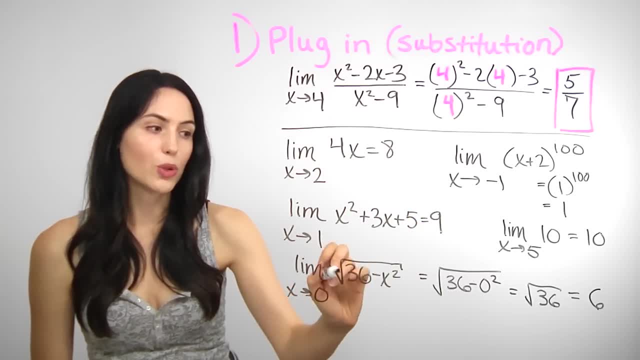 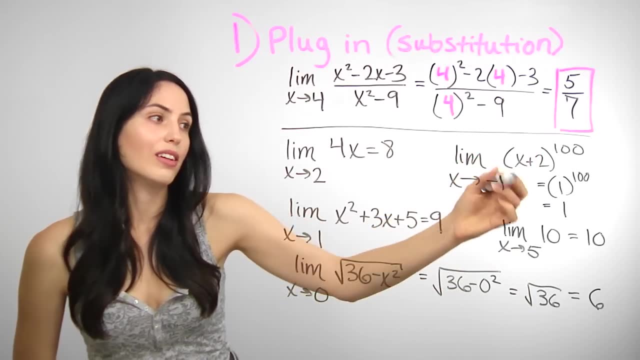 by plugging in any polynomial you can plug into square root of something that ends up being a square root of a positive number or square root of zero, something to a power or limit of a constant. a number is just that number. 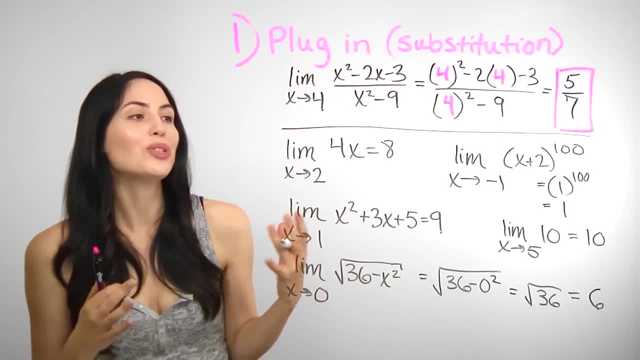 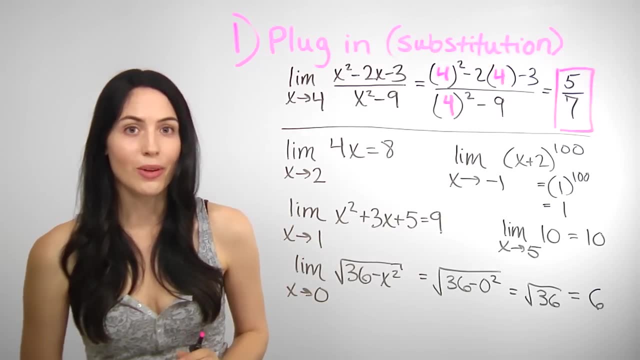 just that constant. Those are all great, but usually finding a limit is not this simple. You might see this once out of 20 times. Usually you'll have to use another way. So let me show you the next way of finding a limit. 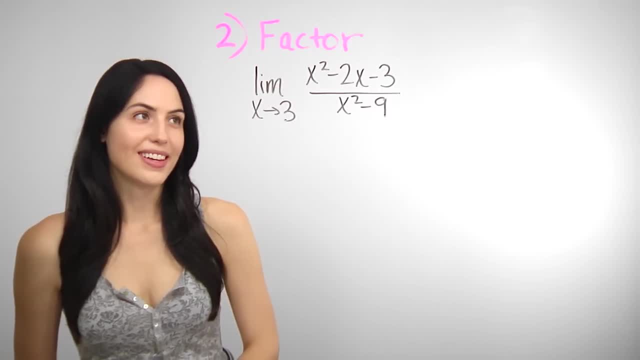 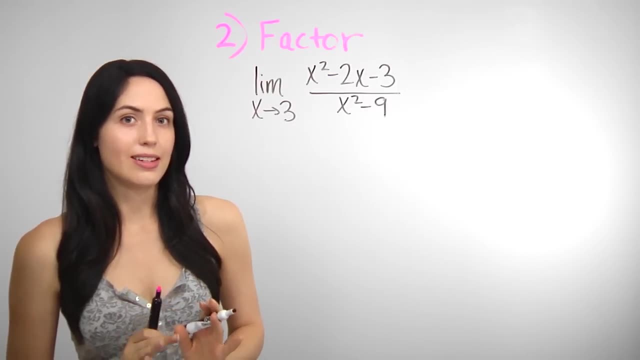 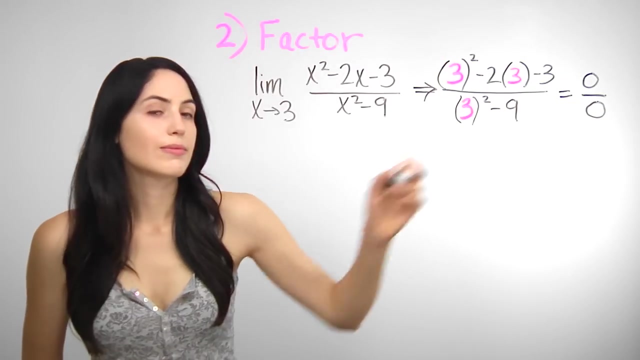 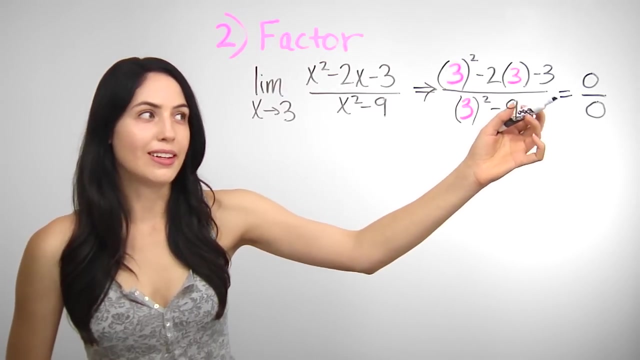 OK, so new problem, but still, the first thing you should try to find the limit is to plug in and see if you get a finite number, a finite value. All right, so you've plugged in and you did not get a finite number like 2 or 10.. 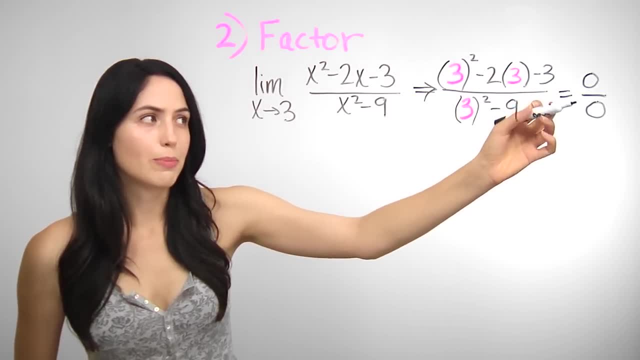 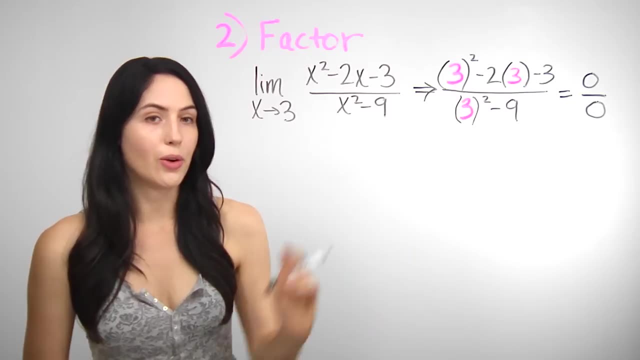 You got not only a 0 in the denominator, which is problematic, But 0 over 10.. 0 over 0, the indeterminant form. If you get 0 in the denominator or 0 over 0, that is not your limit. 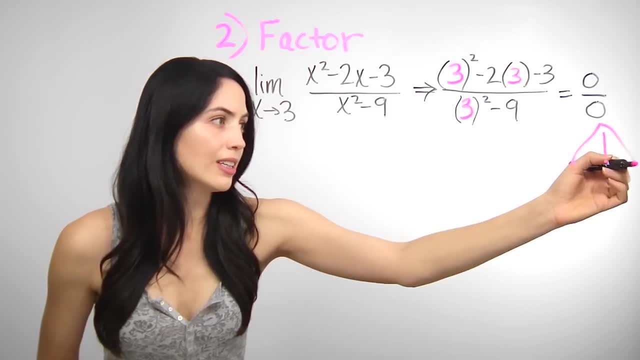 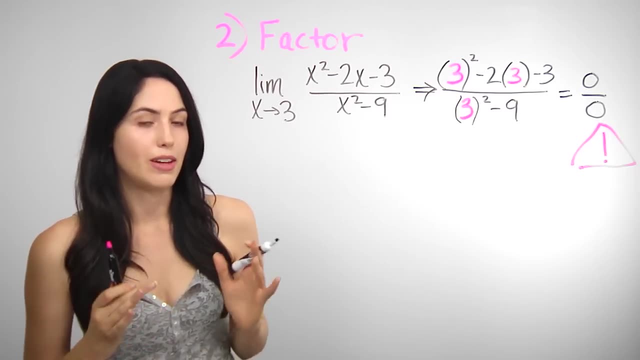 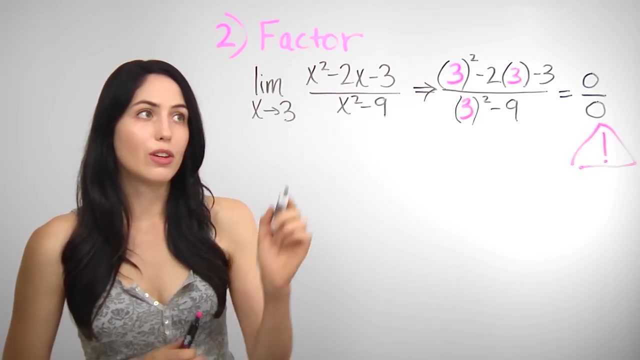 So caution warning, that is not your limit, You are not done. It actually is a sign to you that you need to try something else to find your limit number, limit value. And the next best thing to try is factoring, especially if your function expression has polynomial. 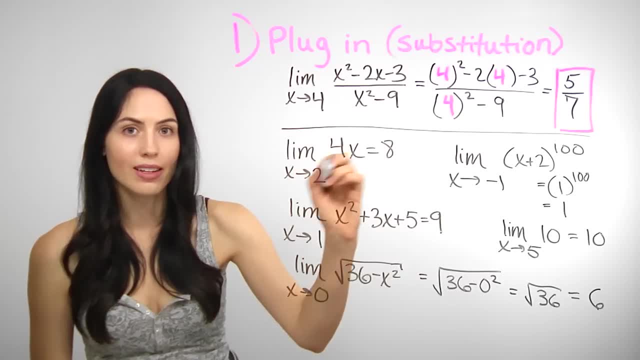 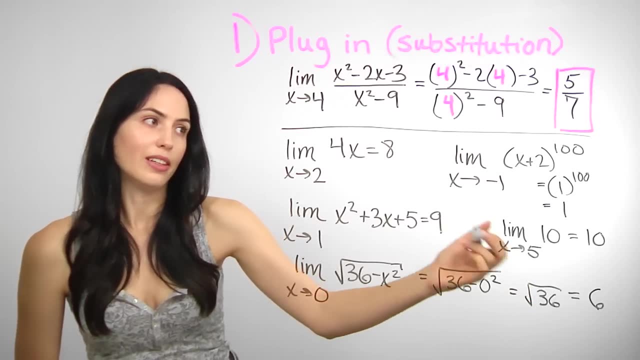 These are all other limits you can find just by plugging in. by plugging in any polynomial you can plug into square root of something. that ends up being a square root of a positive number or square root of zero. something to a power. 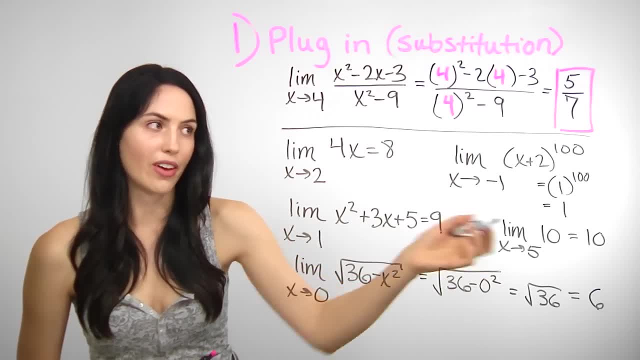 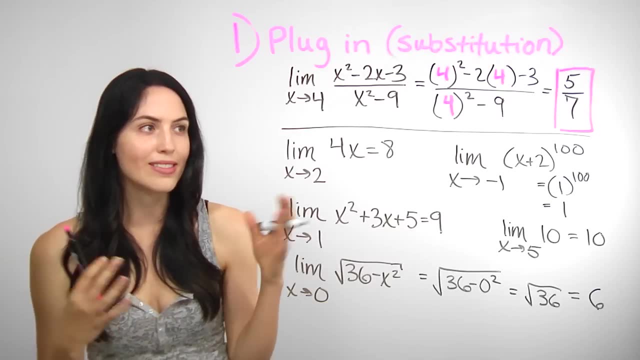 or limit of a constant. a number is just that number, just that constant. Those are all great, but usually finding a limit is not this simple. You might see this once out of 20 times. Usually you'll have to use another way. 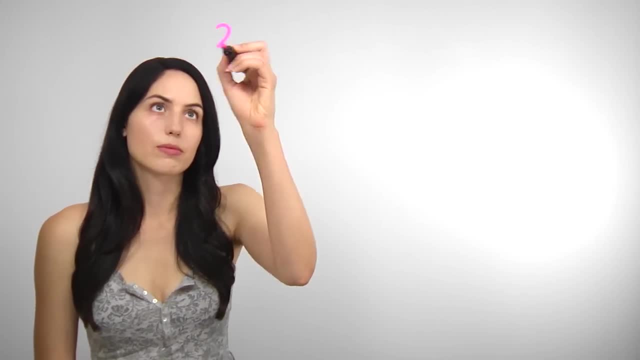 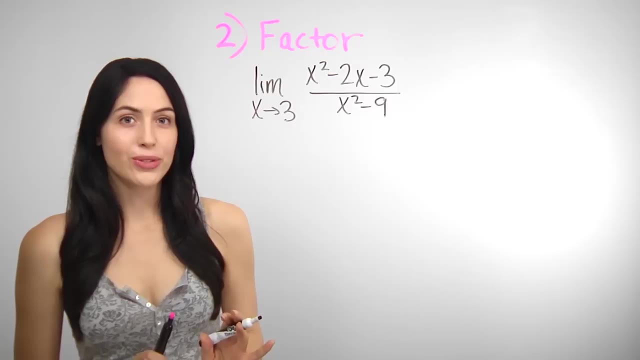 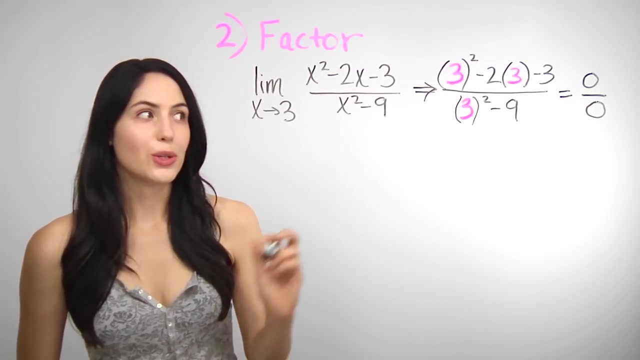 So let me show you the next way of finding a limit. OK, so new problem, but still, the first thing you should try to find the limit is to plug in and see if you get a finite number, a finite value. All right, so you've plugged in and you did not. 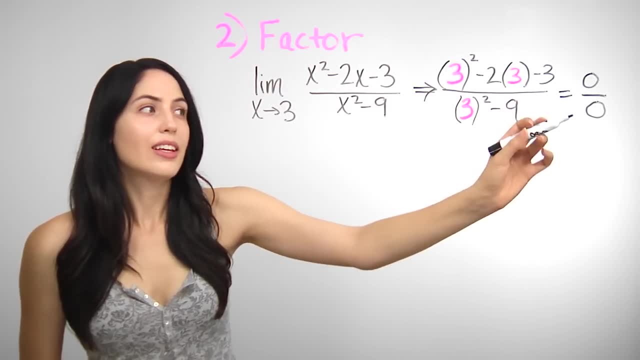 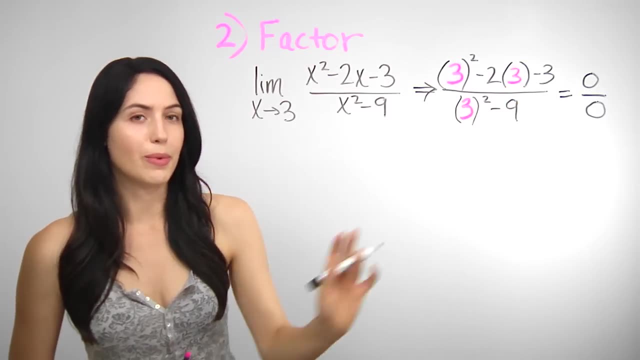 get a finite number like 2 or 10.. You got not only a 0 in the denominator, which is problematic, But 0 over 10.. 0 over 0, the indeterminant form, If you get 0 in the denominator or 0 over 0,. 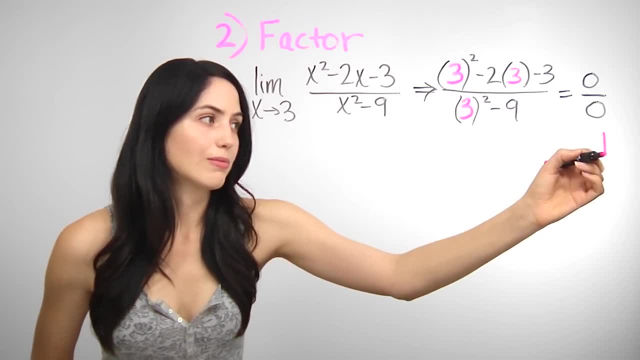 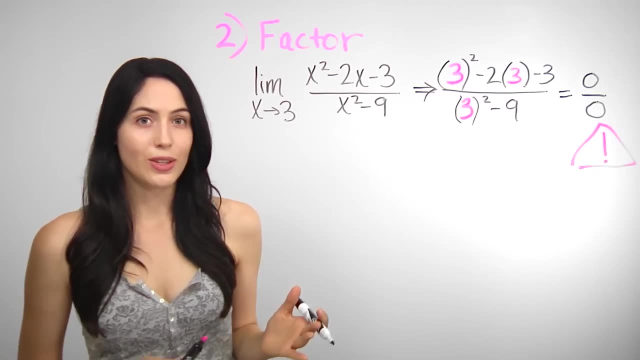 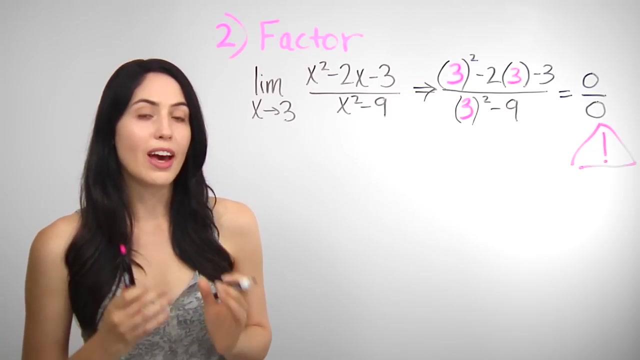 that is not your limit. So caution warning, that is not your limit. You are not done. It actually is a sign to you that you need to try something else to find your limit number, limit value, And the next best thing to try is factoring. 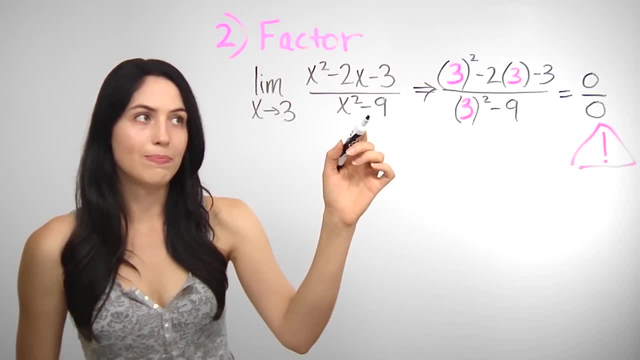 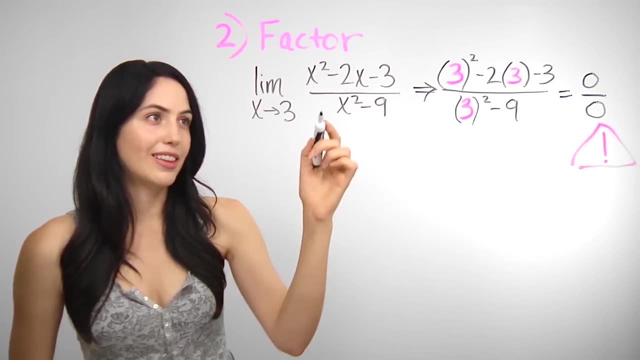 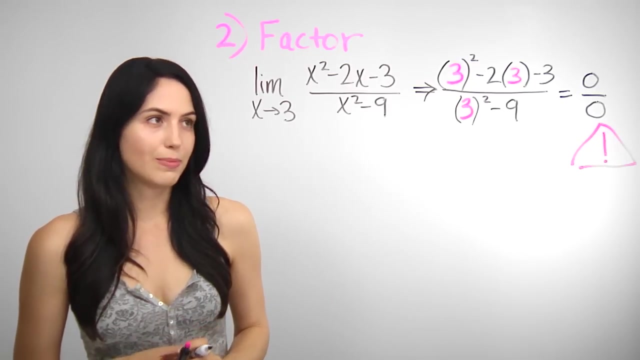 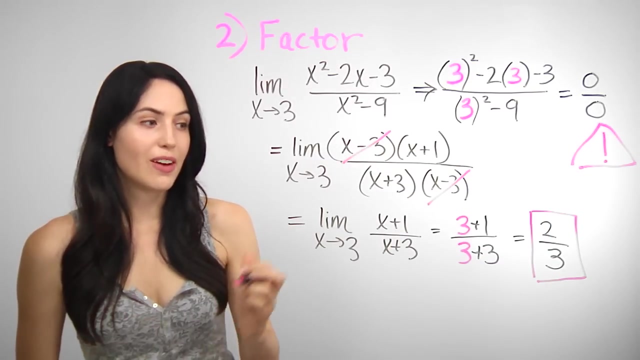 especially if your function expression has polynomial. So this one is begging for you to try factoring it. There's a difference of squares in the bottom, There's a quadratic on top, So you want to try to factor it. This is great, because after factoring, 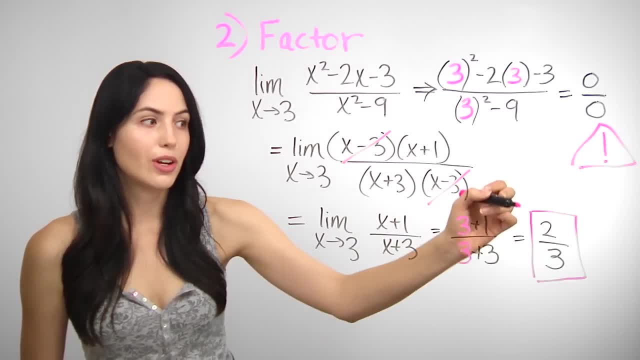 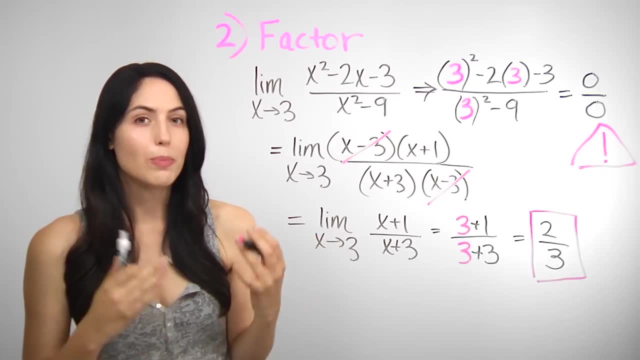 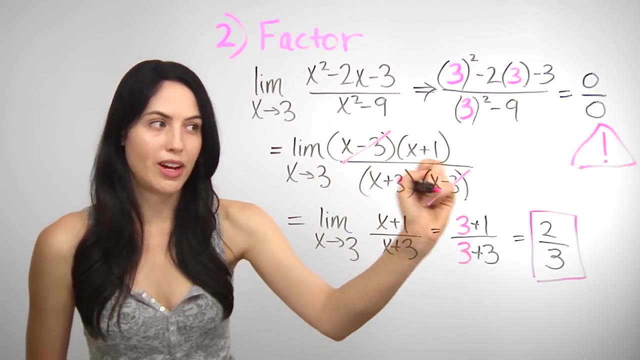 we were able to plug in and get an actual number, finite number, 2 thirds, as the limit value. The limit is equal to 2 thirds. Why did this work? The point of factoring was that it got rid of these problem terms: x minus 3 over x minus 3, those terms that were creating 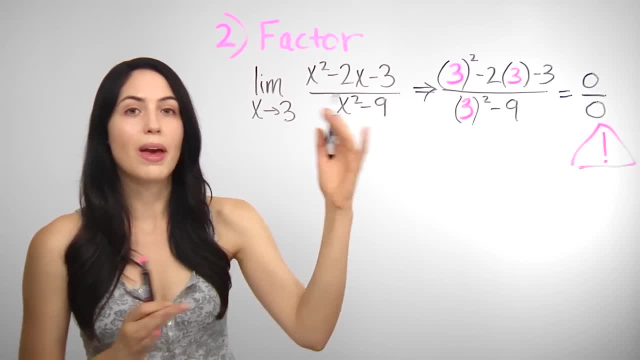 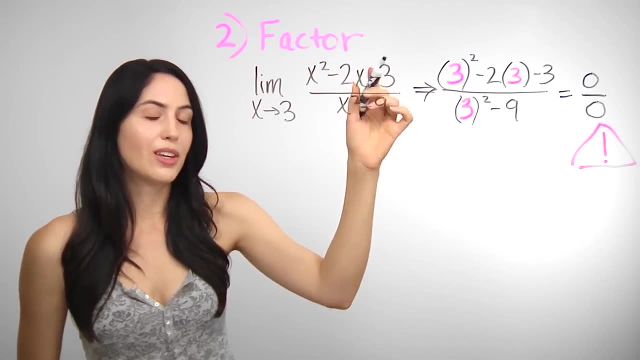 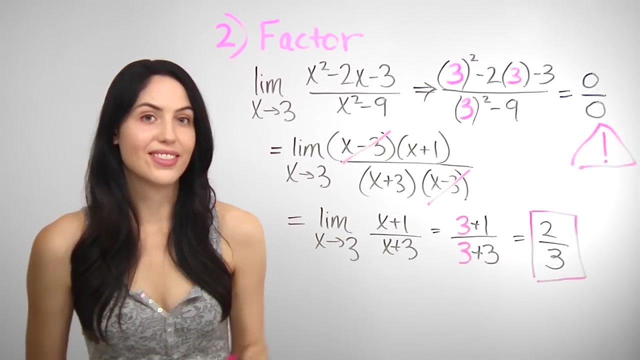 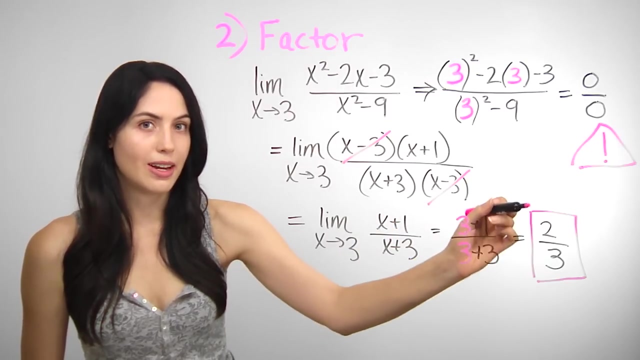 So this one is begging for you to try factoring it. There's a difference of squares in the bottom, There's a quadratic on top, So you want to try to factor it. This is great because after factoring we were able to plug in and get an actual number: finite number. 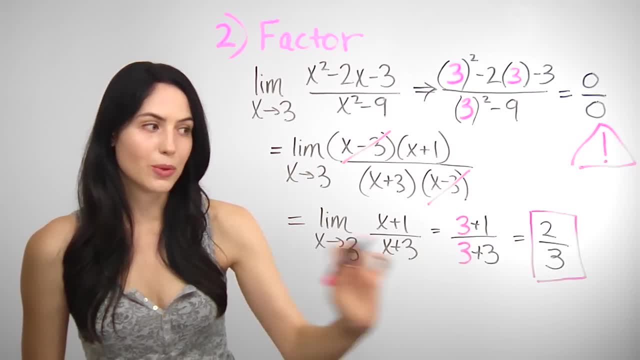 2 thirds as the limit value, The limit is equal to 2 thirds. Why did this work? The point of factoring was that it got rid of these problem terms: x minus 3 over x minus 3, those terms that were creating. 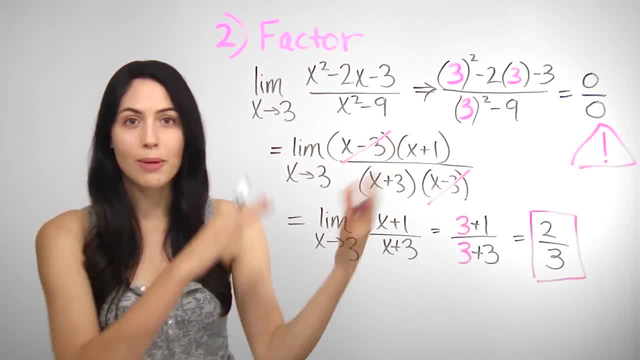 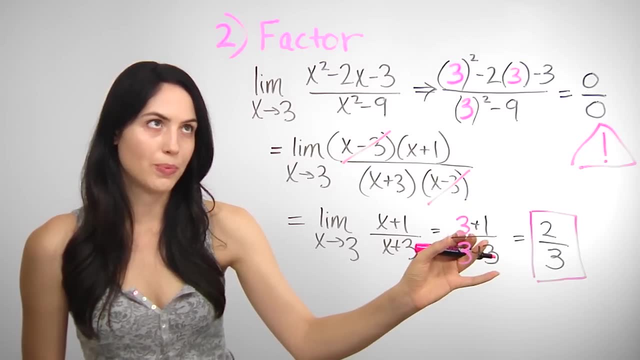 the 0 over 0 form. Now that they're gone, now that they dropped out and they've disappeared, you are able to plug in and really just get the actual number that the limit is equal to. But what happens if you factor and terms, cancel, and then you 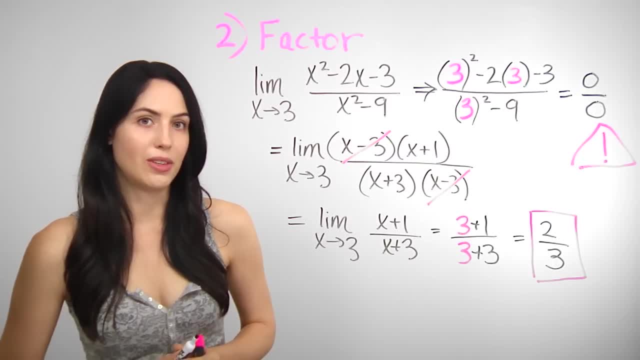 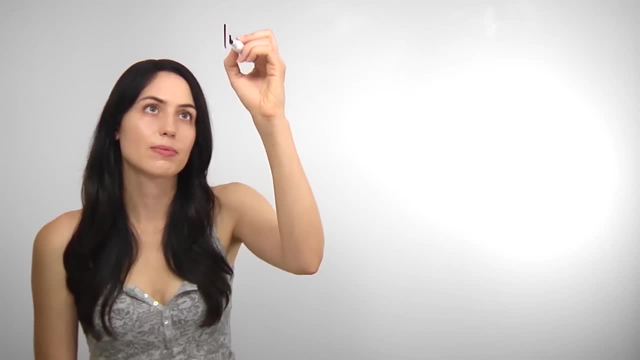 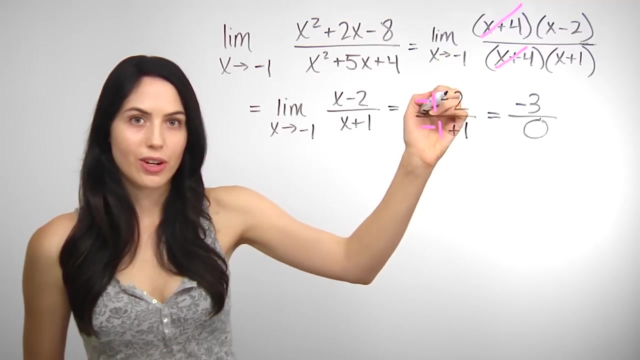 try to plug in. You plug in at the end and you still get 0 in the denominator or, worse, 0 over 0. What then? OK, look at this one. What if you've factored canceled terms? you plug in again. 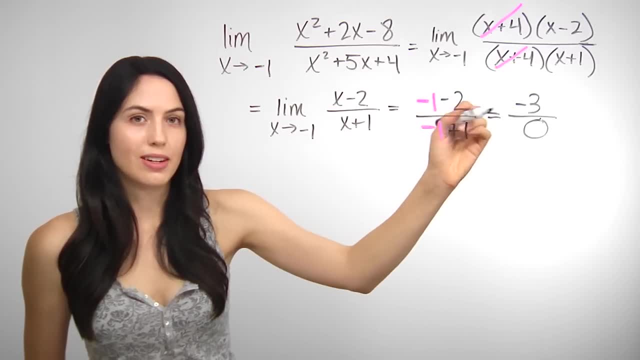 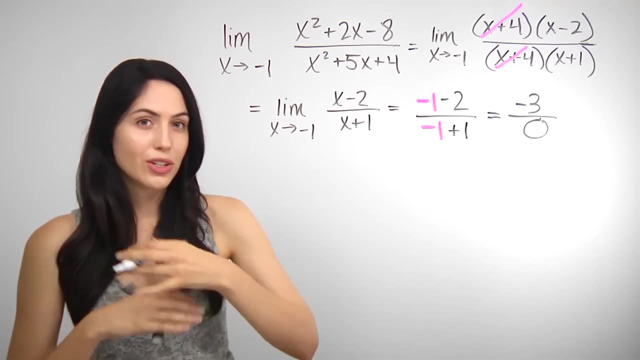 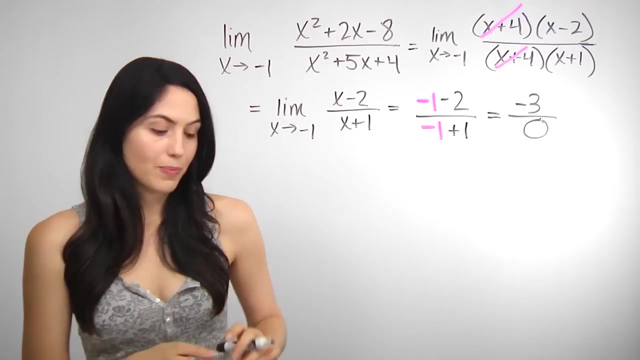 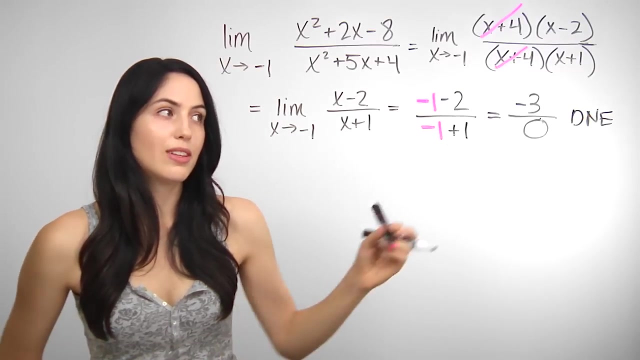 at the end and you still get 0 in the denominator, which is undefined. This means that your function is increasing, is increasing without limit, shooting off to infinity or negative infinity. It's limitless and you can write d and e for the limit. 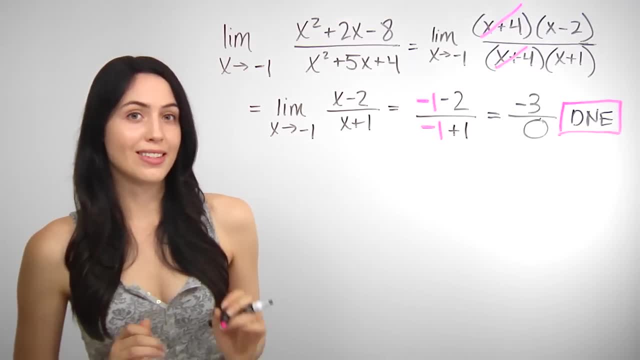 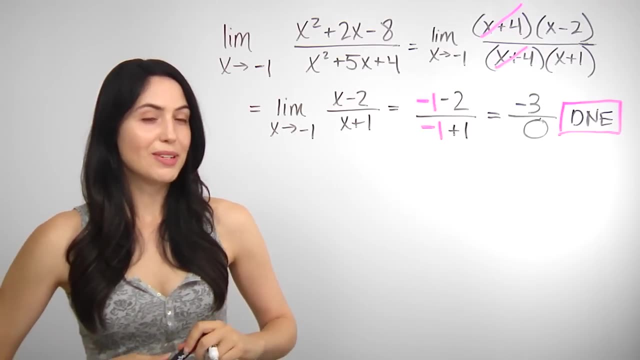 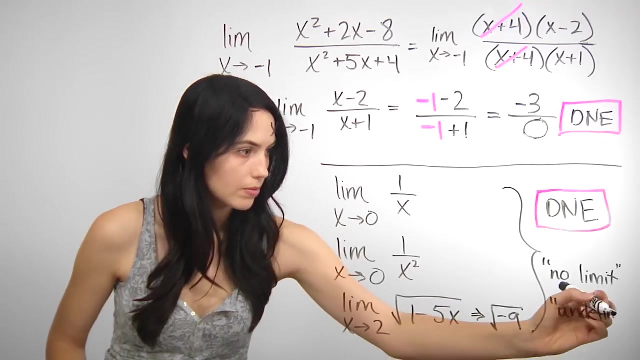 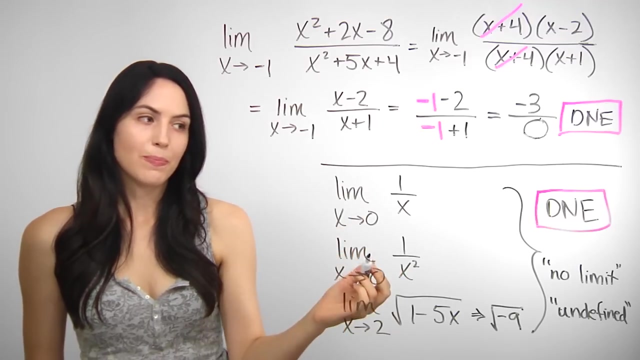 does not exist. The limit does not exist, And if you can remember that, you can be a state champion like the North Shore mathletes. Let me show you some other common types where the limit does not exist. Here are some common function types where the limit does not exist. 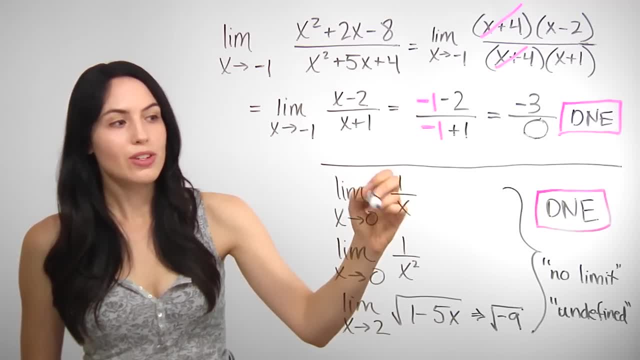 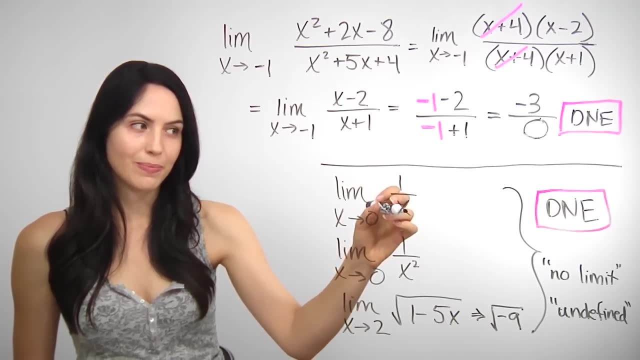 The limit, as x approaches 0, of 1 over x. Here there's nothing else you can do. to simplify the 1 over x, You can't factor anymore, and plugging in 0 gives you an undefined expression. So there is no limit. 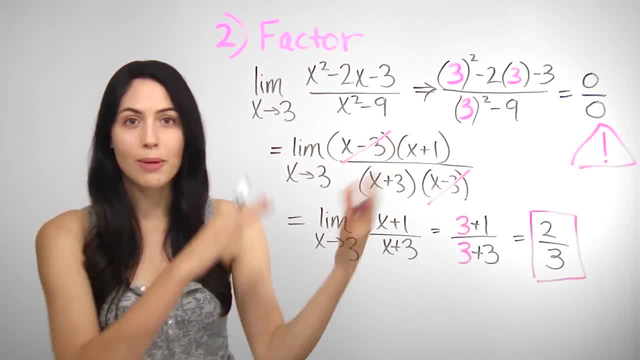 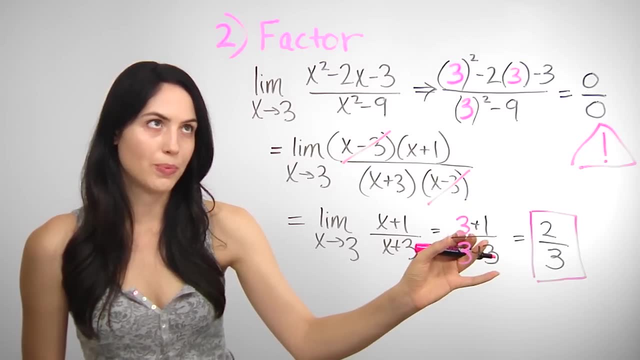 the 0 over 0 form. Now that they're gone, now that they dropped out and they've disappeared, you are able to plug in and really just get the actual number that the limit is equal to. But what happens if you factor and terms, cancel, and then you 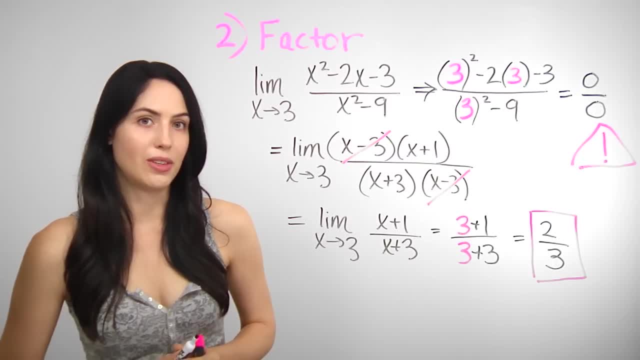 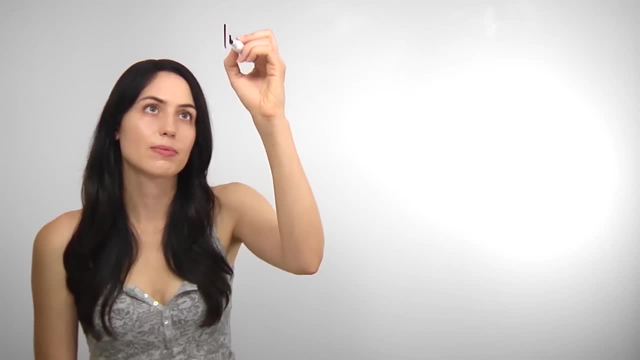 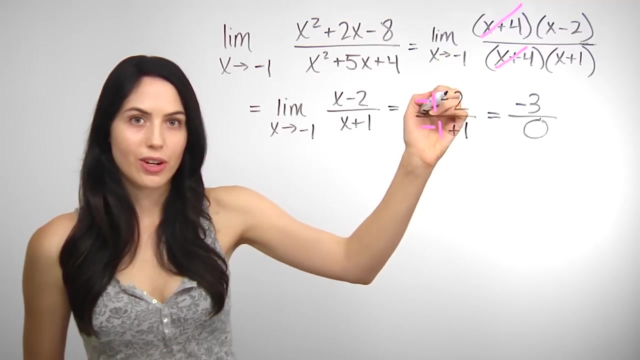 try to plug in. You plug in at the end and you still get 0 in the denominator or, worse, 0 over 0. What then? OK, look at this one. What if you've factored canceled terms? you plug in again. 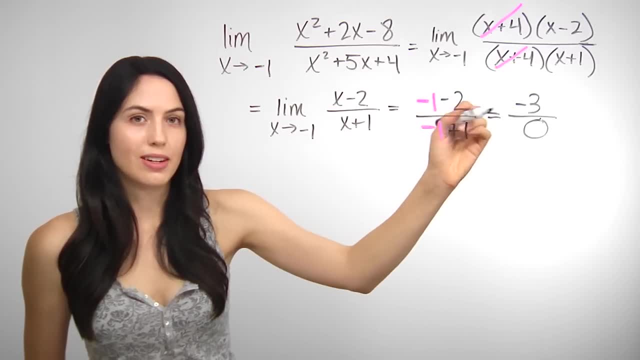 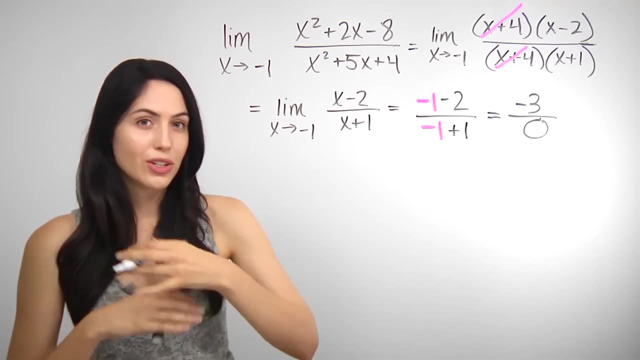 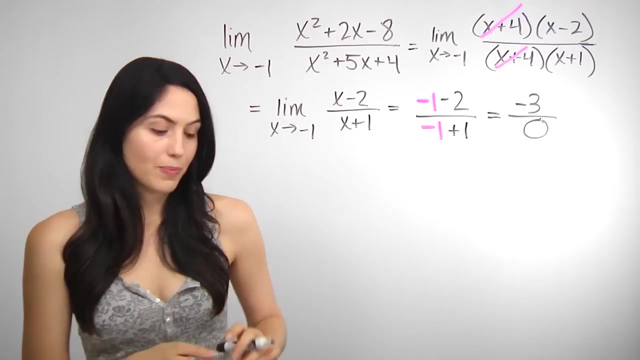 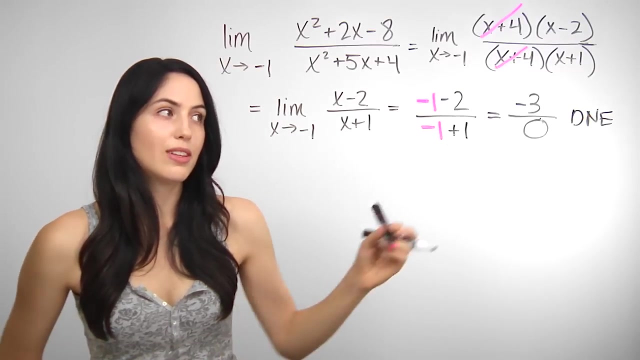 at the end and you still get 0 in the denominator, which is undefined. This means that your function is increasing, is increasing without limit, shooting off to infinity or negative infinity. It's limitless and you can write d and e for the limit. 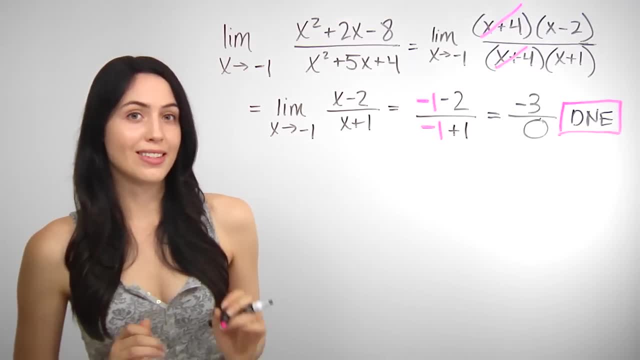 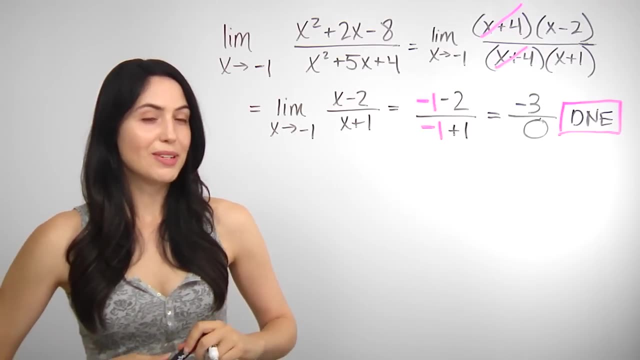 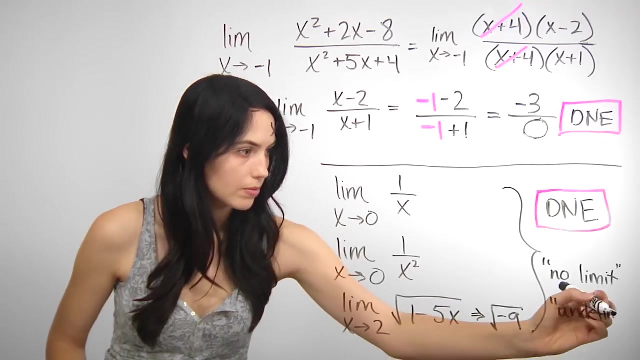 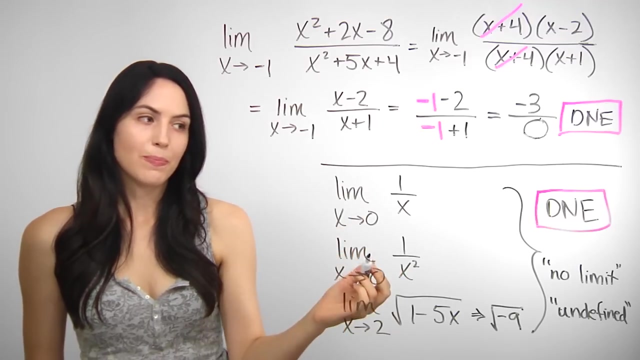 does not exist. The limit does not exist, And if you can remember that, you can be a state champion like the North Shore mathletes. Let me show you some other common types where the limit does not exist. Here are some common function types where the limit does not exist. 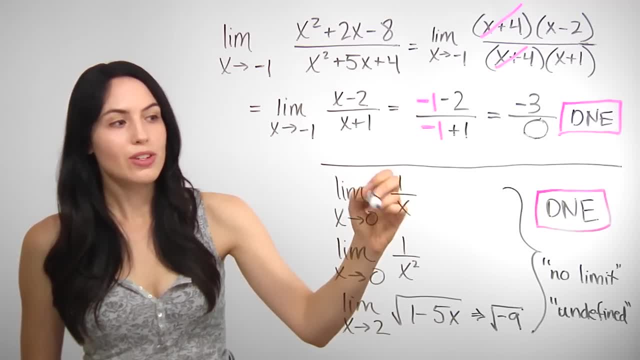 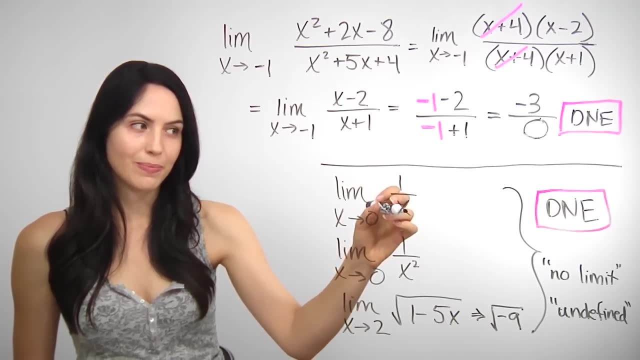 The limit, as x approaches 0, of 1 over x. Here there's nothing else you can do. to simplify the 1 over x, You can't factor anymore, and plugging in 0 gives you an undefined expression. So there is no limit. 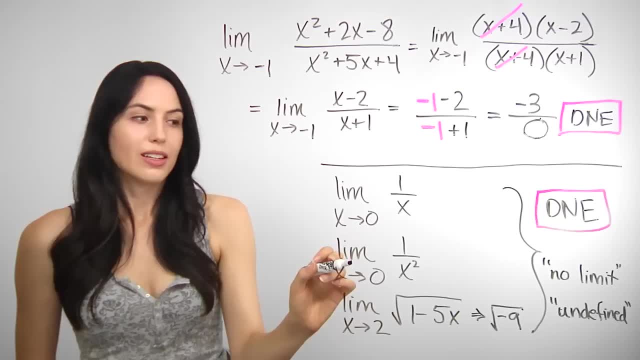 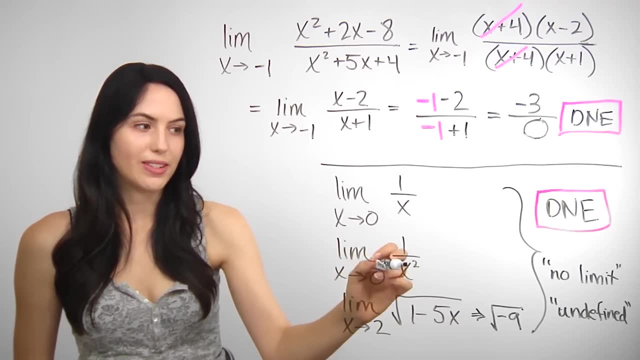 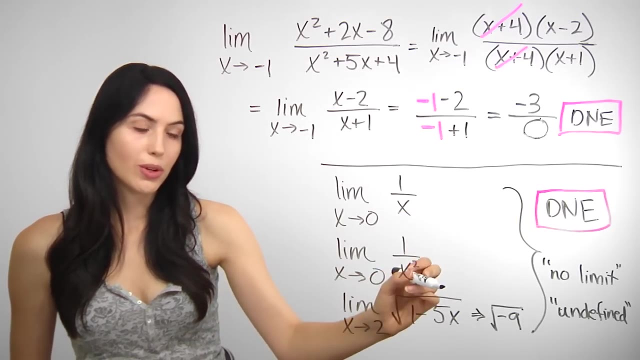 It does not exist. d and e: Similar situation here, The limit as x goes to 0 of 1 over x squared. You can't factor that anymore. This is not defined. There is no limit, It does not exist. Also, here, the square root of something that turns out to be: 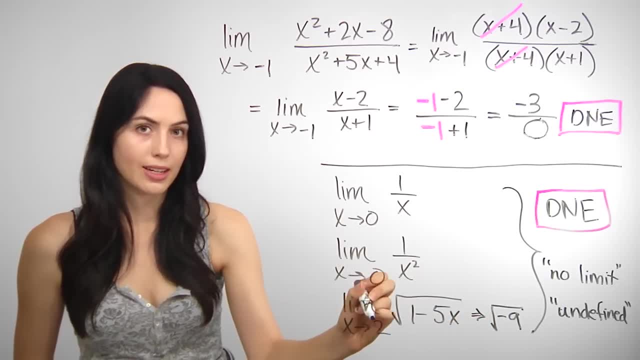 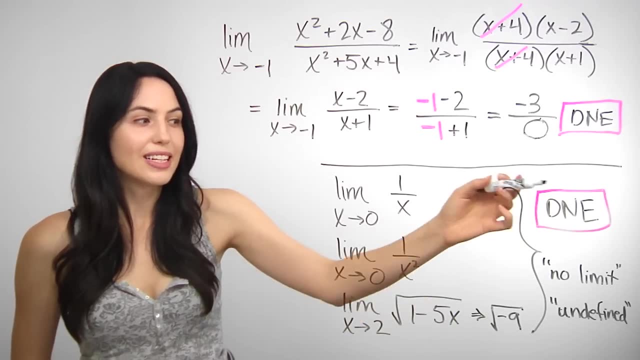 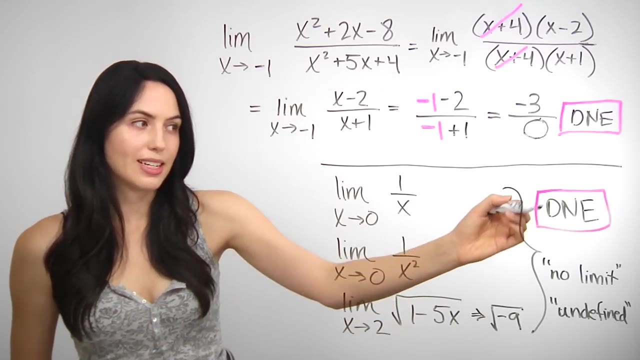 square root of a negative number when you take the limit when you plug in, is not defined. There's no limit. It's also d and e. These all have the same meaning. here, in limit world, You can just write d and e, for the limit does not exist. 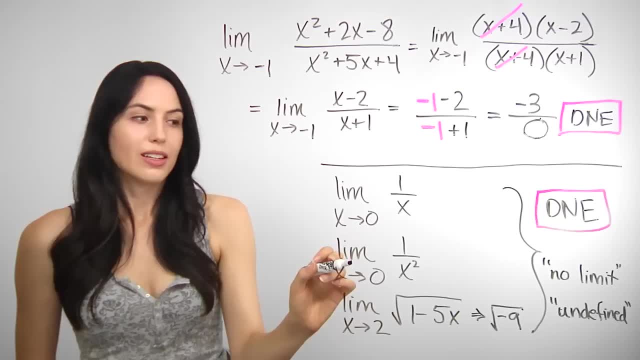 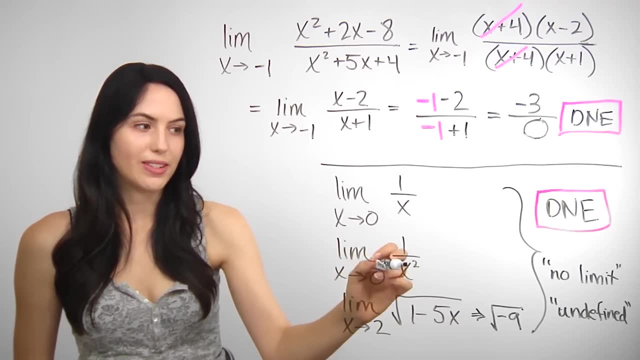 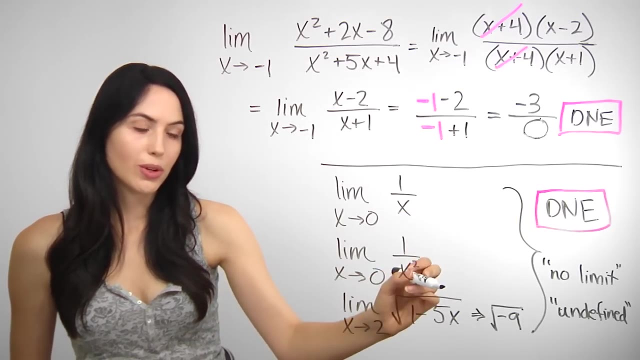 It does not exist. d and e: Similar situation here, The limit as x goes to 0 of 1 over x squared. You can't factor that anymore. This is not defined. There is no limit, It does not exist. Also, here, the square root of something that turns out to be: 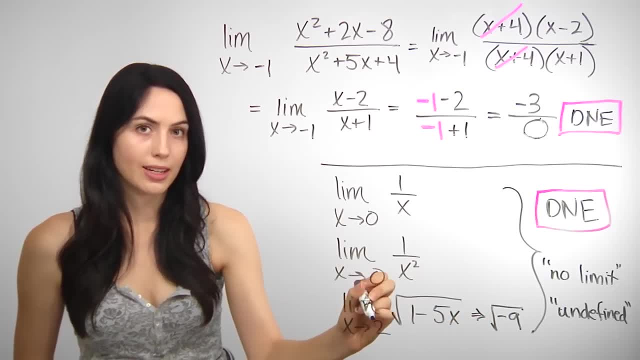 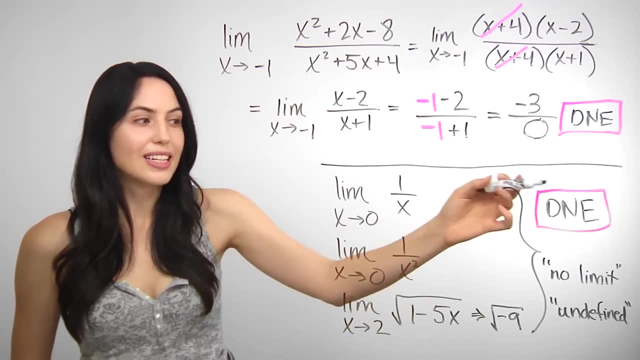 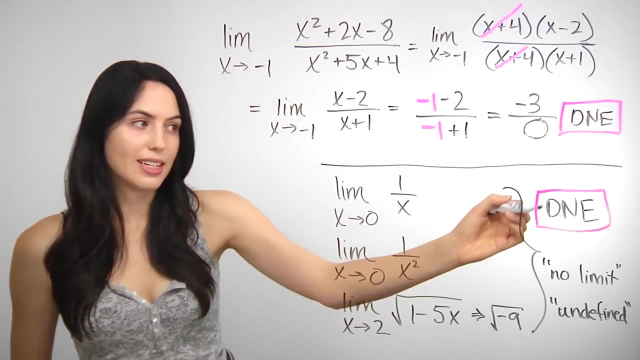 square root of a negative number when you take the limit when you plug in, is not defined. There's no limit. It's also d and e. These all have the same meaning. here, in limit world, You can just write d and e, for the limit does not exist. 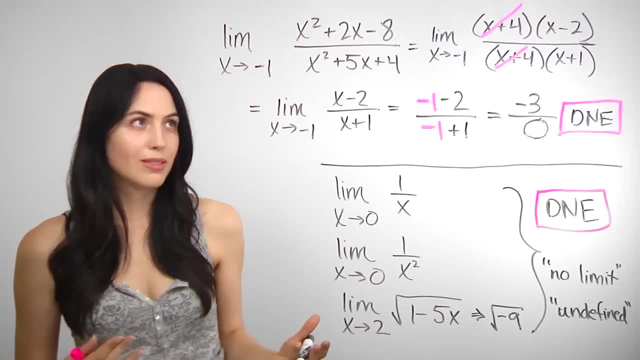 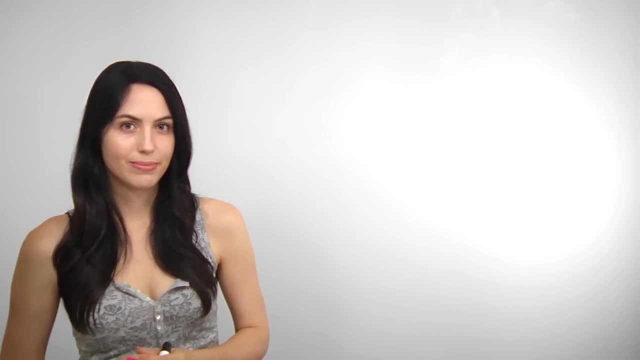 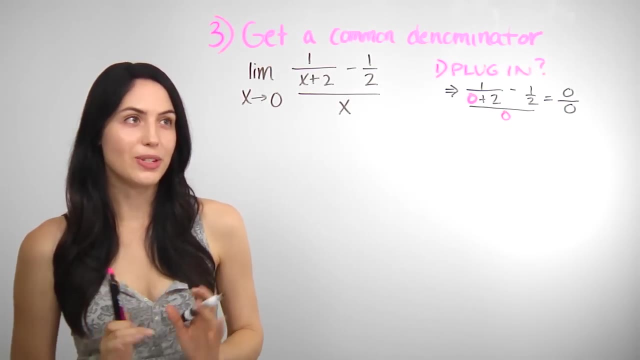 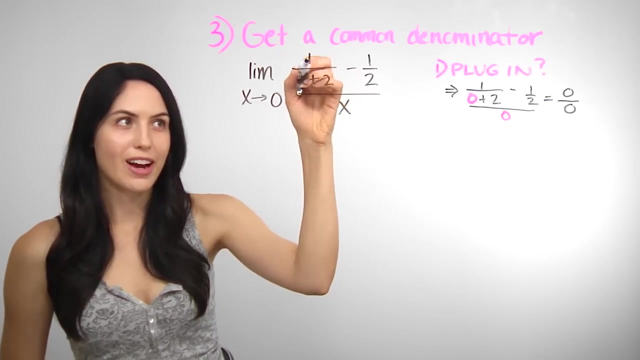 So what if you can't factor as a strategy? There are other things you can try. So let me show you the next best thing to try to find the limit. Okay, a new type. Here we have the limit as x approaches 0 of this expression, which is basically a fraction within a fraction. 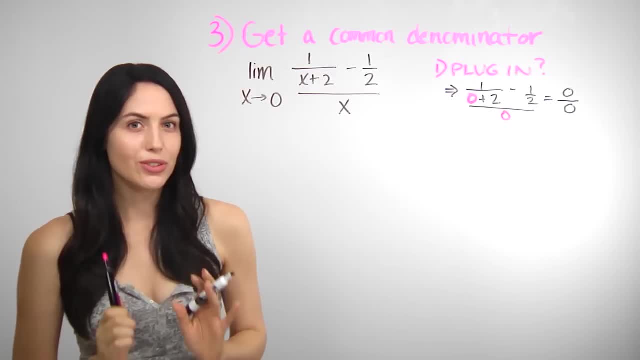 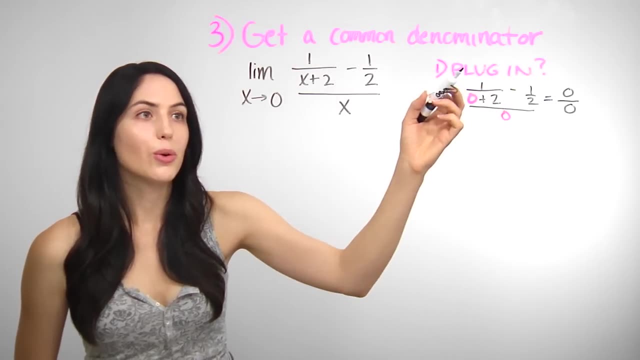 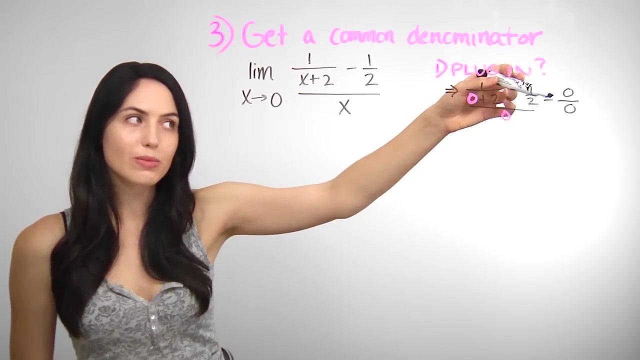 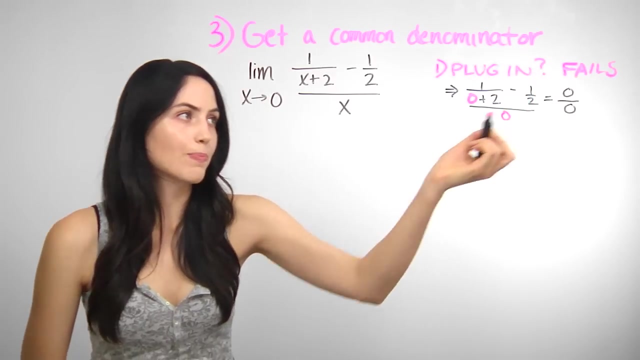 Still, you should still first try the two other steps. you know the two other techniques: Plug in, see if it works. When you do plug in, unfortunately you get zero over zero, the indeterminant form. So plugging in failed. but the second thing to try, remember, is to see if you can factor. 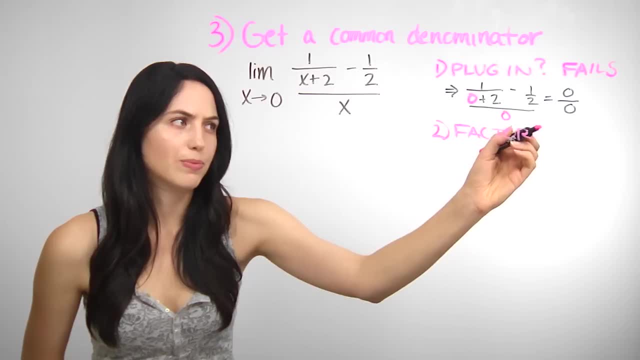 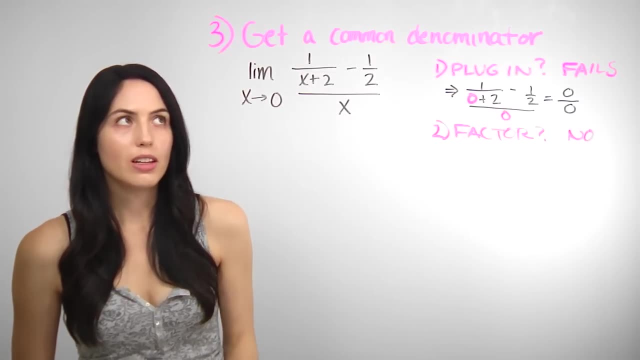 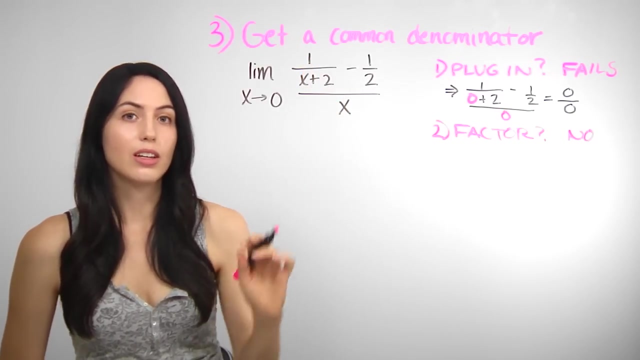 if you look at this expression, there's nothing you can really factor there. so no, then what can you try next? Well, especially if you have something that looks like this, which is a complex rational expression- a fraction within a larger fraction- try to get a common denominator, because then 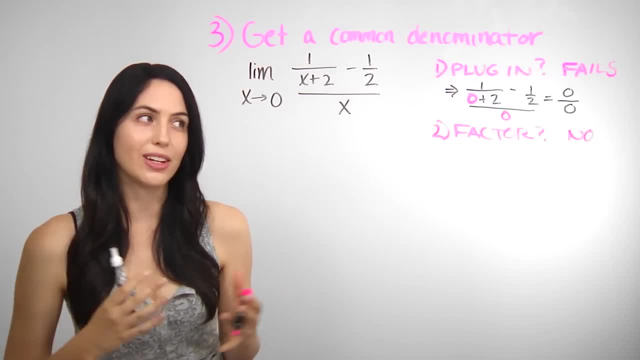 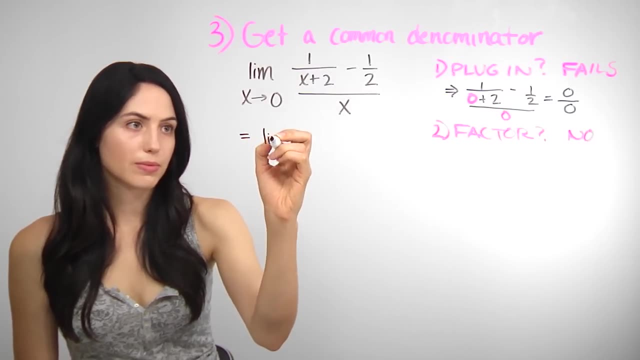 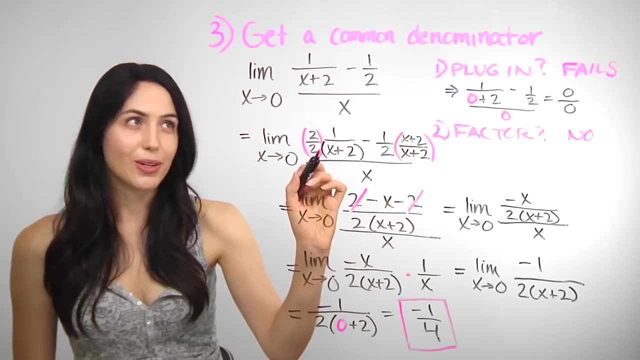 things will simplify, some things will magically cancel and you will be able to probably plug in and get your limit value. Okay, let's look at this work. So you need to get a common denominator so that you can combine these fractions up here. 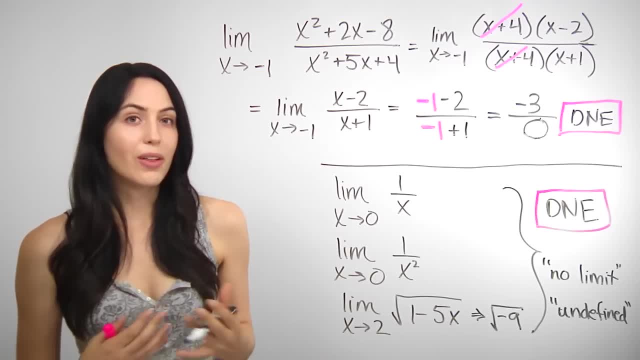 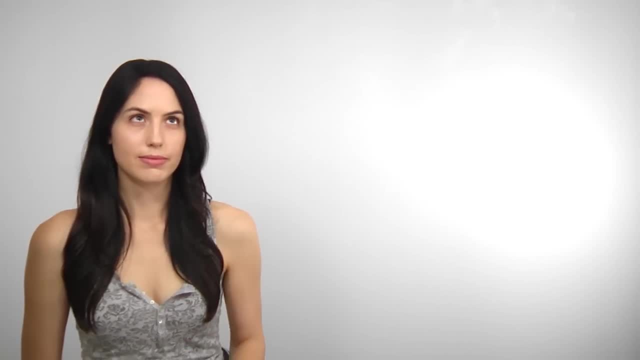 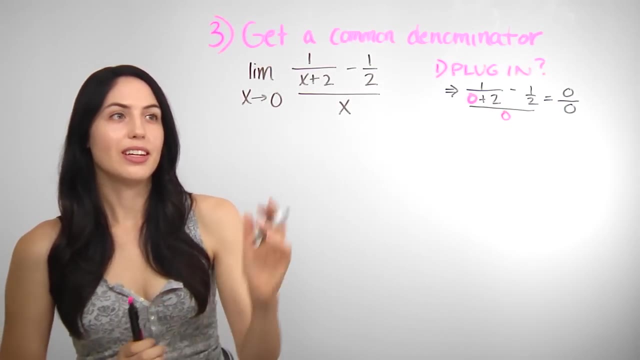 What if you can't factor as a strategy? There are other things you can try. Let me show you the next best thing to try to find the limit. OK, a new type. Here we have the limit as x approaches 0 of this expression, which is basically a fraction. 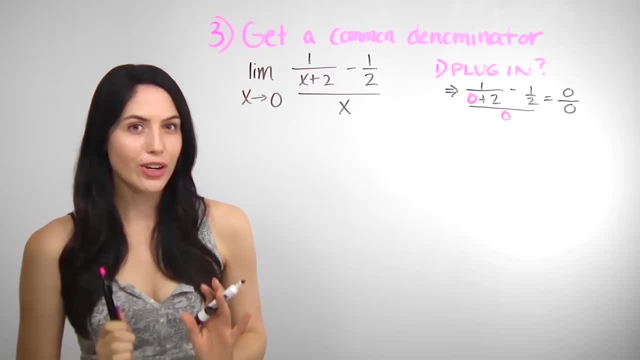 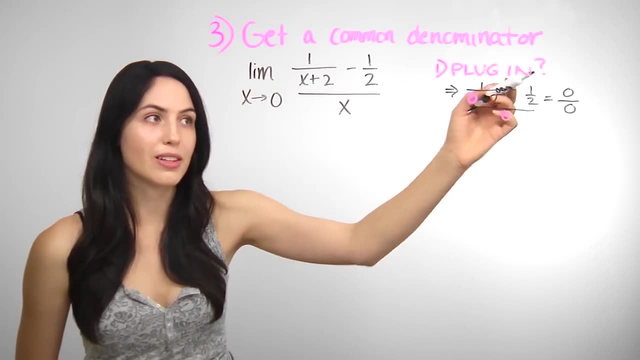 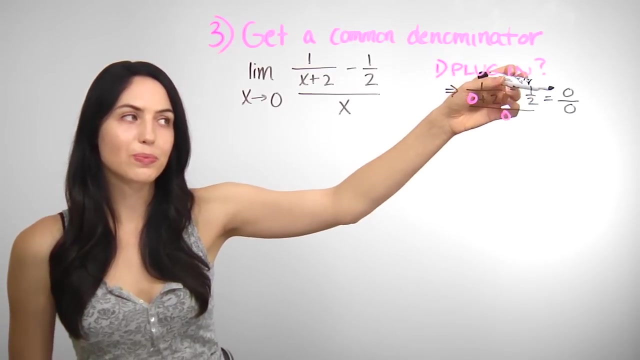 than a fraction. Still, you should still first try the two other steps. you know the two other techniques: Plug in, see if it works. When you do plug in, unfortunately, you get zero over zero, the indeterminate form. So 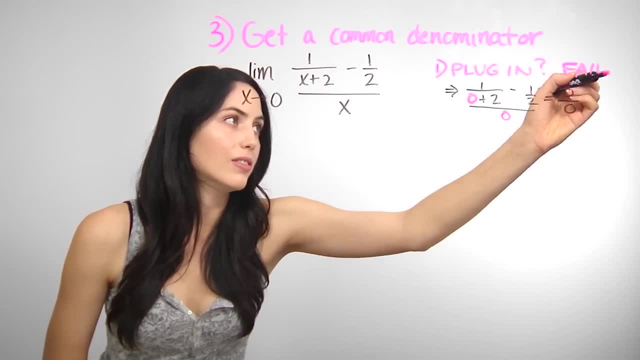 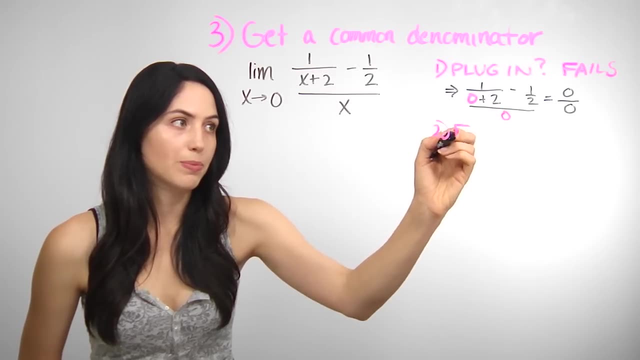 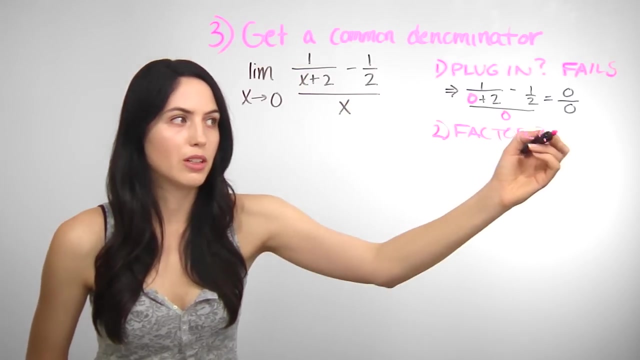 plugging in failed Fails. But the second thing to try remember is to see if you can factor. If you look at this expression, you really there's nothing you can really factor there. so no, Then what can you try next? 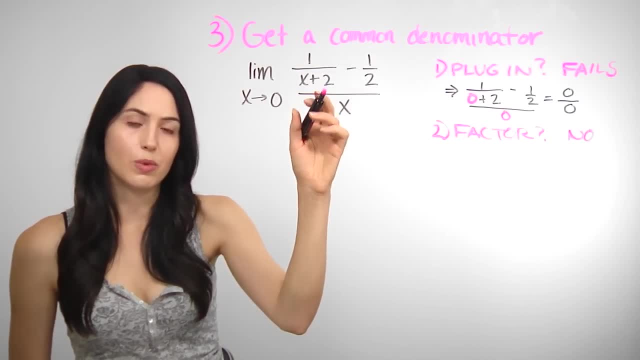 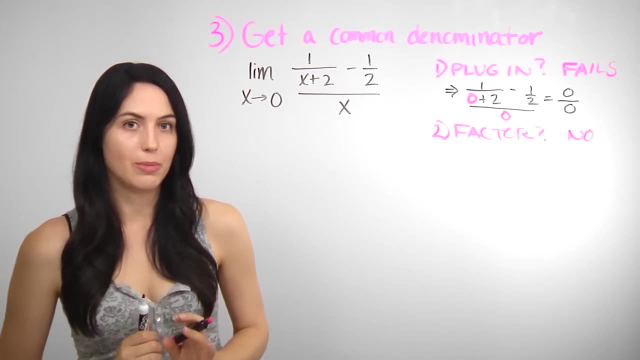 Well, especially if you have something that looks like this, which is a complex rational expression, a fraction within a larger fraction, try to get a common denominator, because then things will simplify, some things will magically cancel and you will be able to probably plug in and 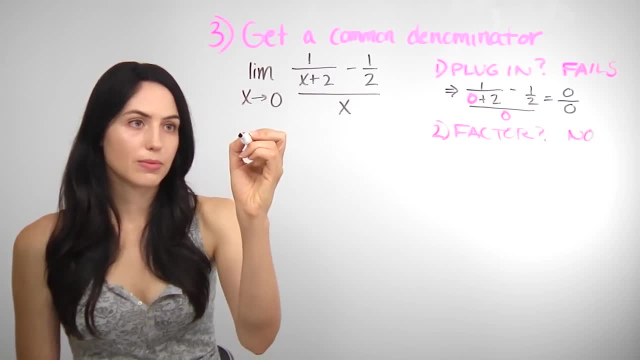 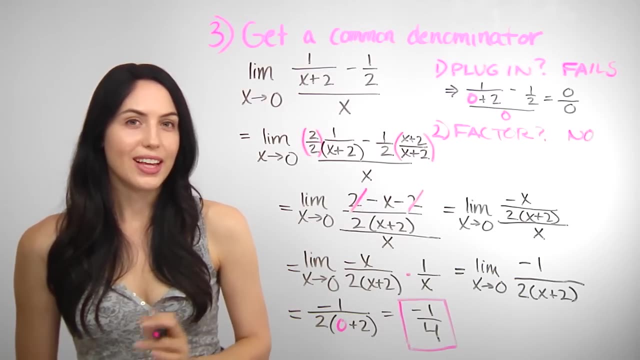 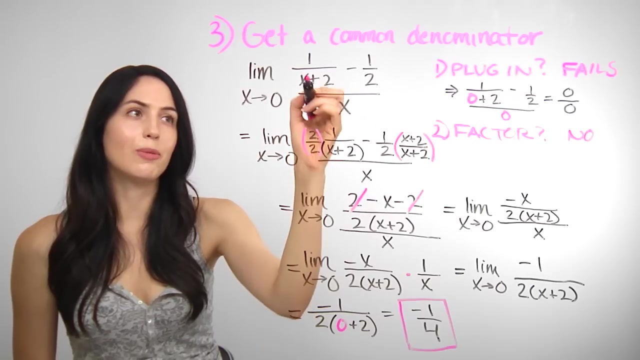 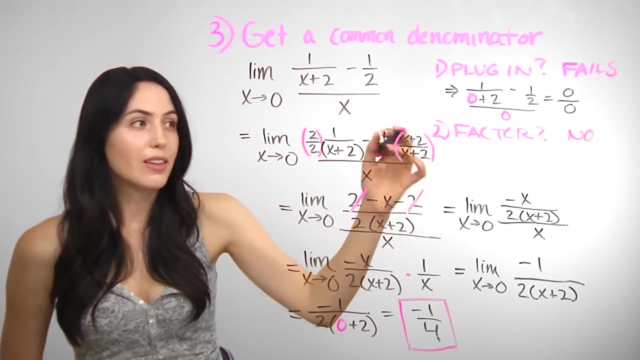 get your limit value. Okay, let's look at this work. So you need to get a common denominator so that you can combine these fractions up here. A common denominator between x plus 2 and 2.. Think about this: Getting a common denominator, factoring the other technique. 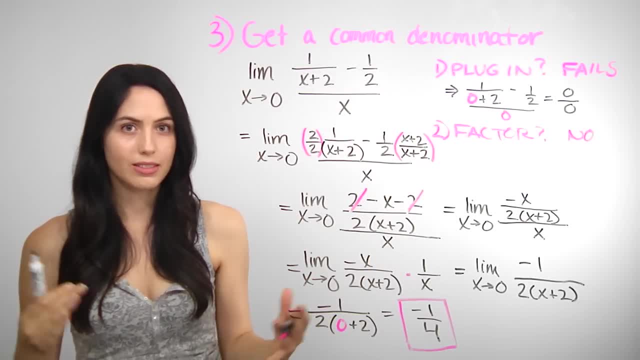 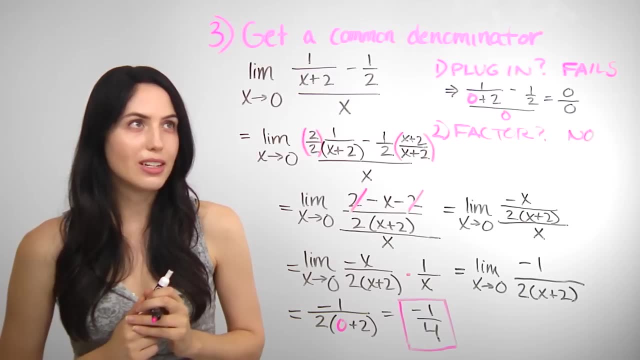 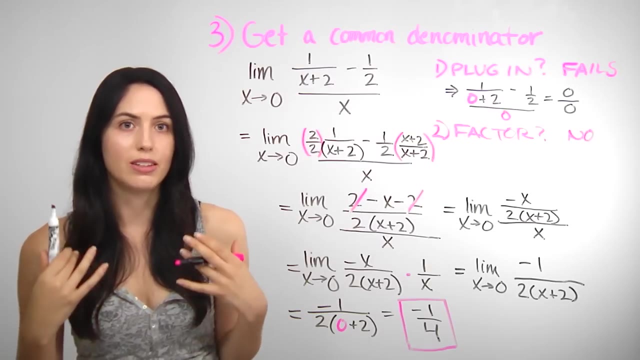 plugging in. these are all just algebra techniques. These are all just algebra techniques that you've seen before. Hopefully you've seen before. Now they've come back to haunt you But they are not so intimidating, hopefully. The real hard part with limits is knowing which method to use, which way to find a limit. 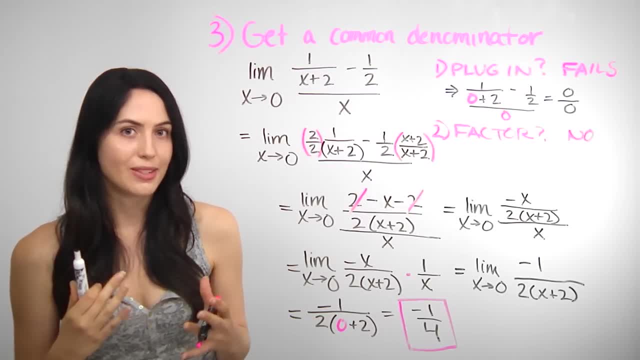 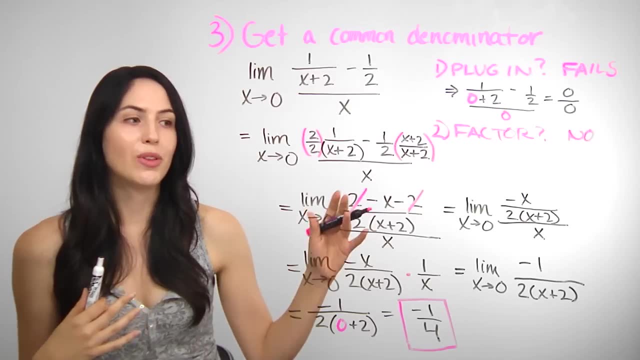 And what I'm really hoping to give you in this video is kind of an order, a structure in your mind to make sense of this, so that if someone throws a random limit problem at you, you have an idea of where to start and what to try. And these are some of the most. 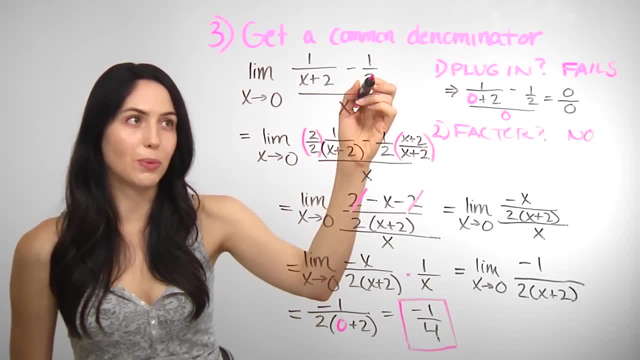 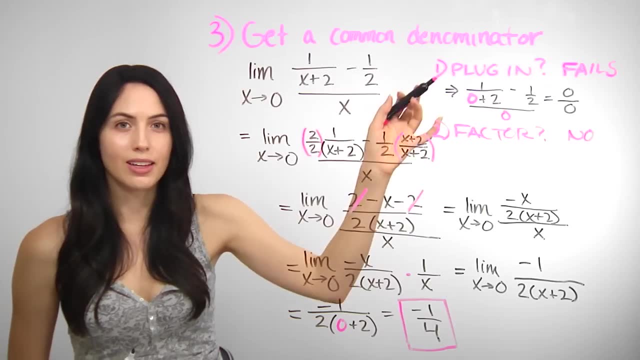 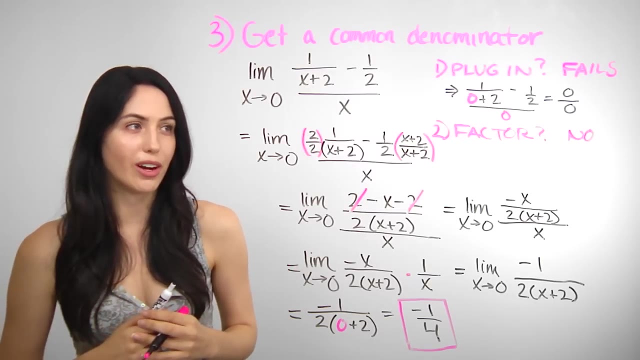 a common denominator between x plus 2 and 2.. Think about this: getting a common denominator, factoring the other technique, plugging in. these are all just algebra techniques that you've seen before, Hopefully You've seen before. now they've come back to haunt you. 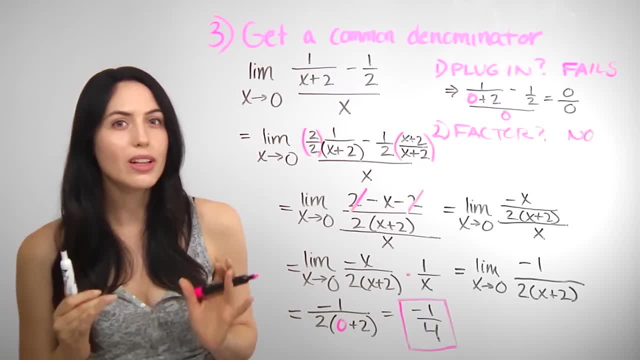 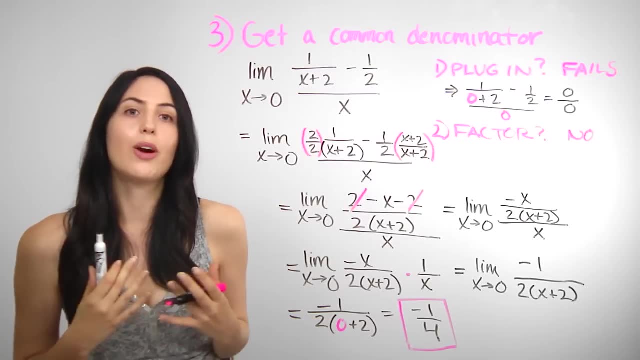 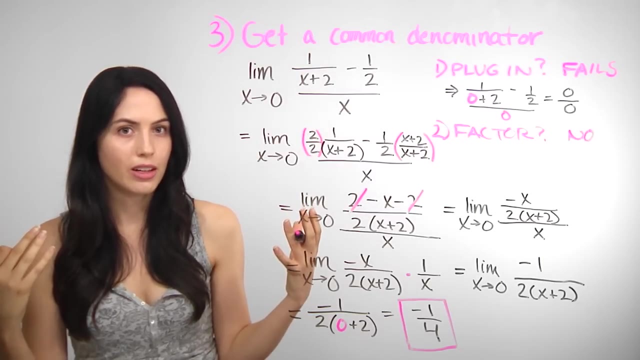 But they are not so intimidating, hopefully. The real hard part with limits is knowing which method to use, which way to find a limit, And what I'm really hoping to give you in this video is kind of an order, a structure in your mind to make sense of this, so that if someone throws a random limit, problem at. 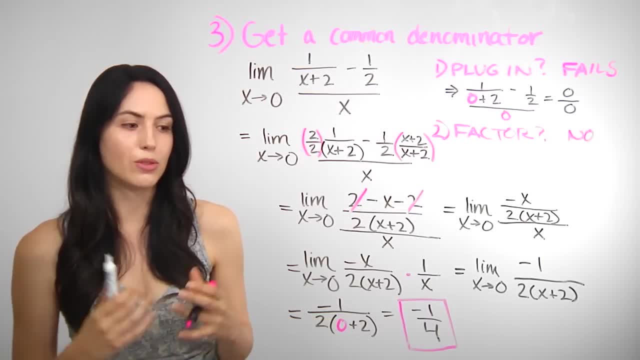 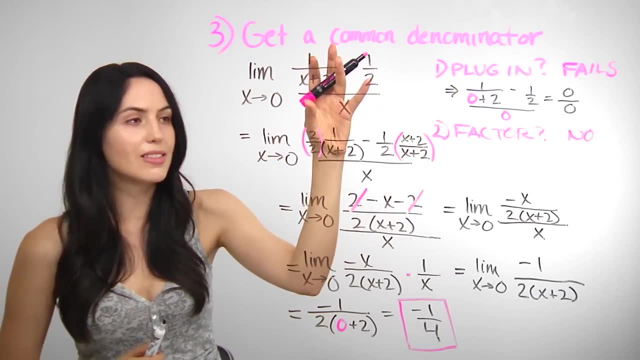 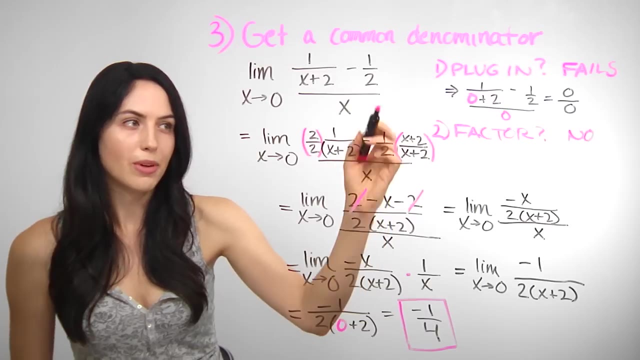 you. you have an idea of where to start and what to try, And these are some of the most common ways of finding limits. So this is a big one. Get a common denominator, especially if it looks like this, And in this case, I just want to remind you of some algebra things that come up: 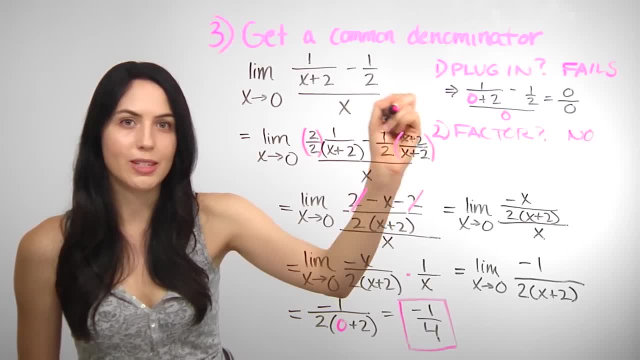 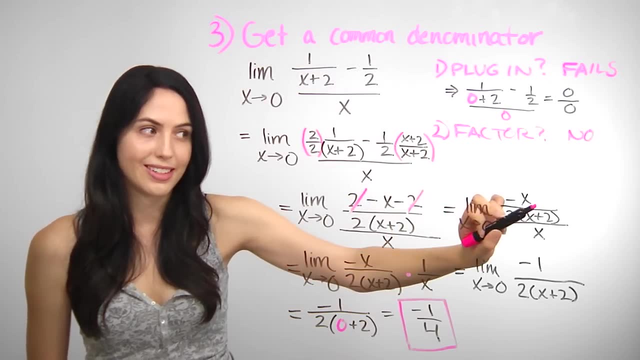 Just remember to distribute a negative sign to both terms within parentheses when you expand. Constant may cancel. In this case, we're left with a negative x over your LCD. your common denominator- Your common denominator is x, So you're left with a negative x over your common denominator. 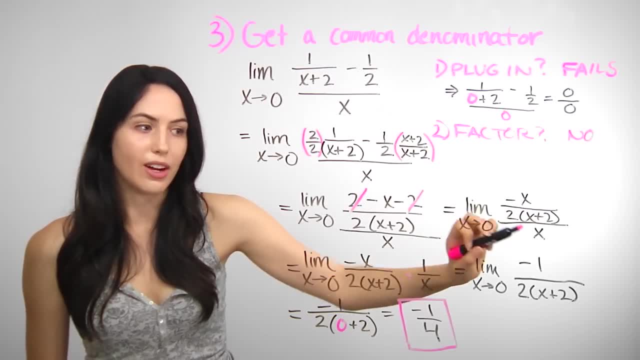 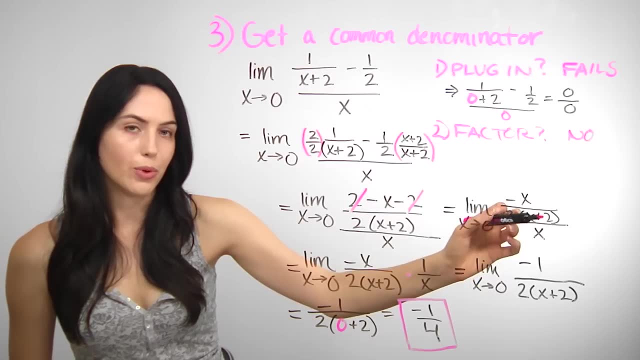 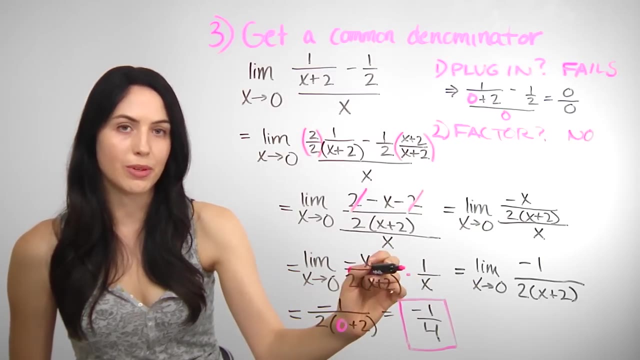 Okay, And your common denominator is 2 times x plus 2, all over x. This will help you simplify. Remember that dividing by a number or a term is the same as multiplying by the reciprocal of that. This will help you simplify. So dividing by x is the same as multiplying by 1 over x. 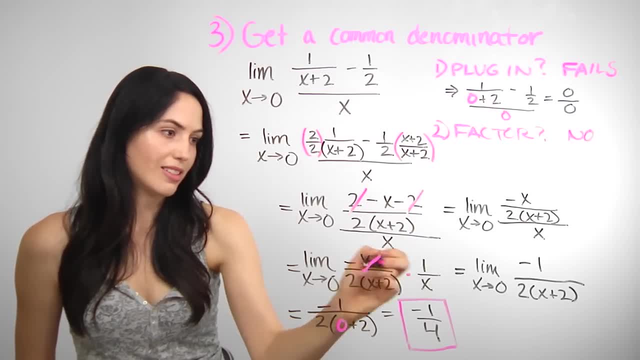 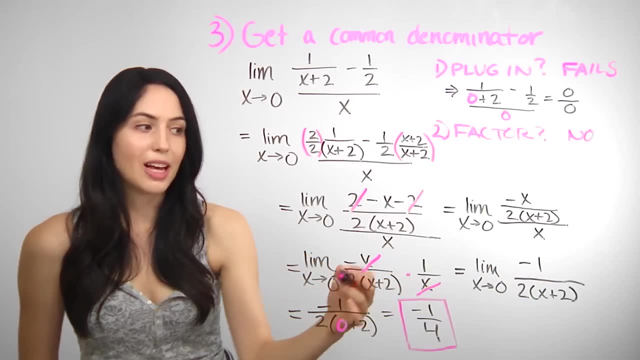 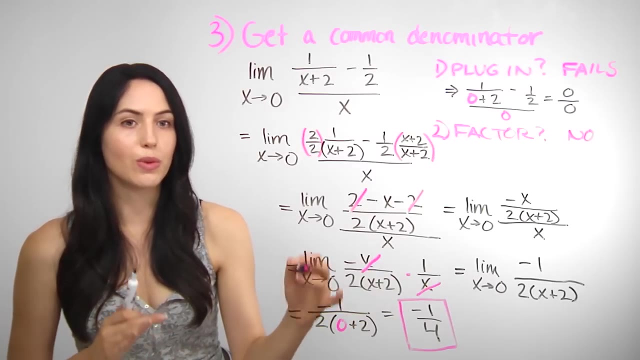 That lets you cancel another term, x and x, so that you have negative 1 over your common denominator. Okay, And then at that point you really are just able to plug in 0 and get an actual number, an actual finite value: negative 1. fourth, 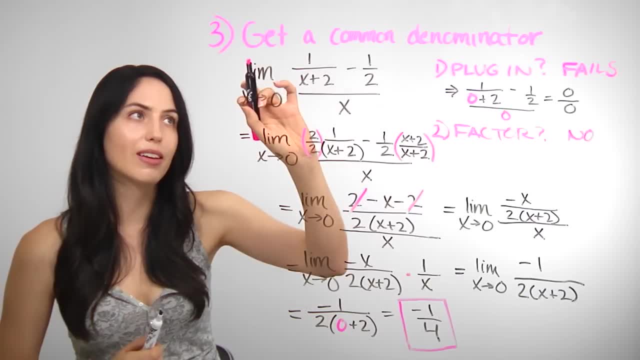 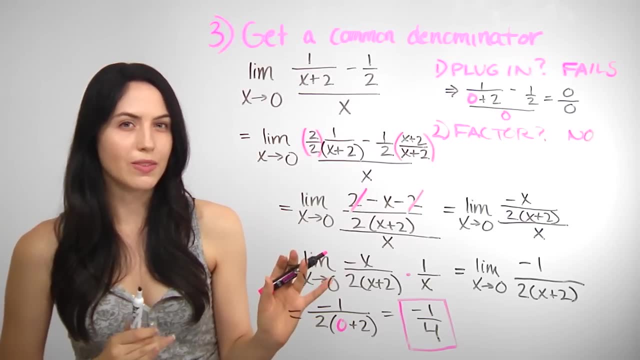 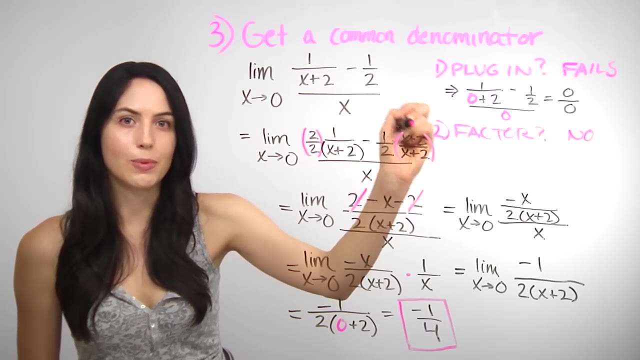 common ways of finding limits. So this is a big one. Get a common denominator, especially if it looks like this, And in this case I just want to remind you of some algebra things that come up. Just remember to distribute a negative sign to both terms within parentheses. 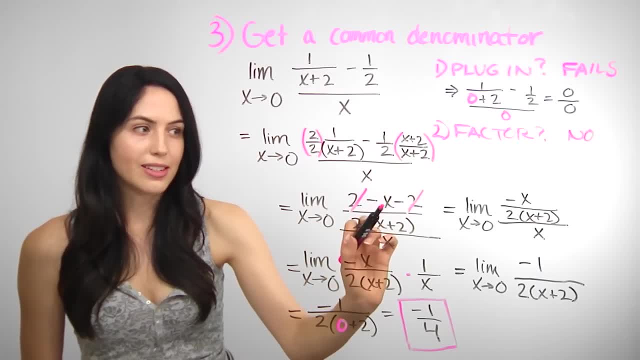 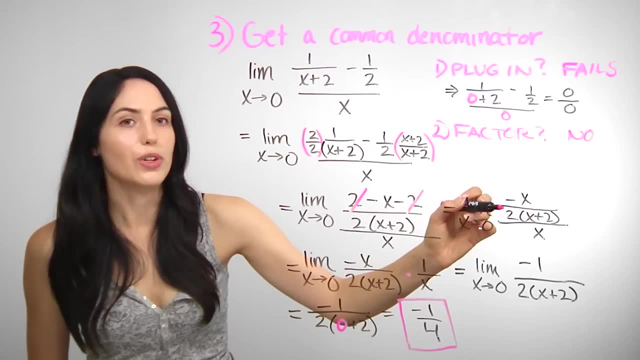 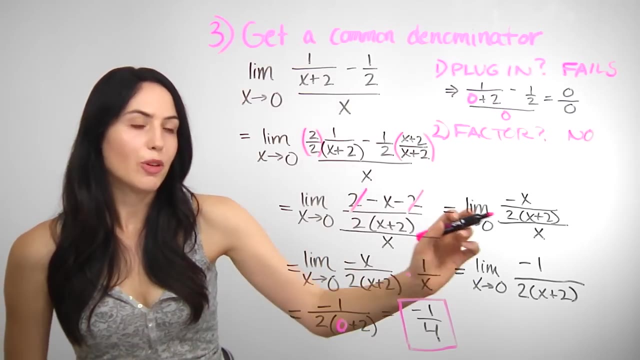 when you expand, Constant may cancel. In this case, we're left with a negative x over your LCD. your common denominator, Your common denominator, is 2 times x plus 2, all over x. This will help you simplify. Remember that dividing by a number or a term is the same as multiplying by the reciprocal. 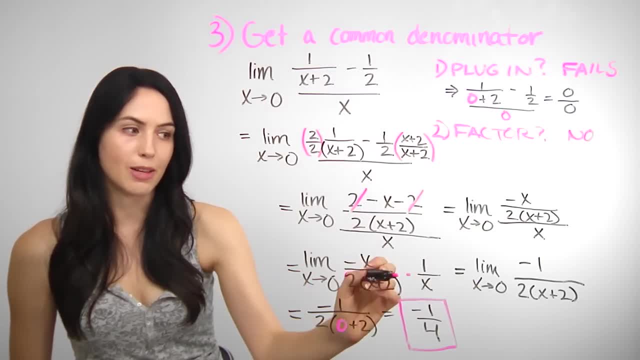 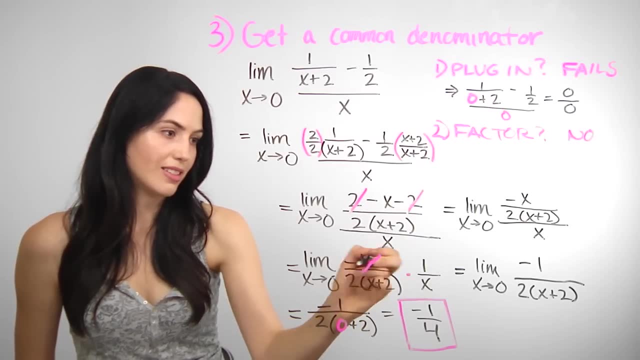 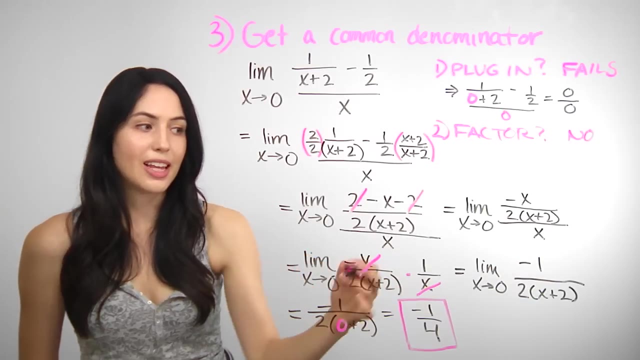 of that. This will help you simplify. So dividing by x is the same as multiplying by 1 over x. That lets you cancel another term, x and x, so that you have negative 1 over your x. So you're left with a common denominator, And then at that point you really are just 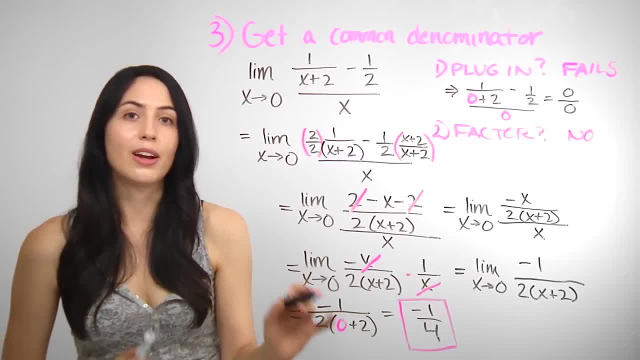 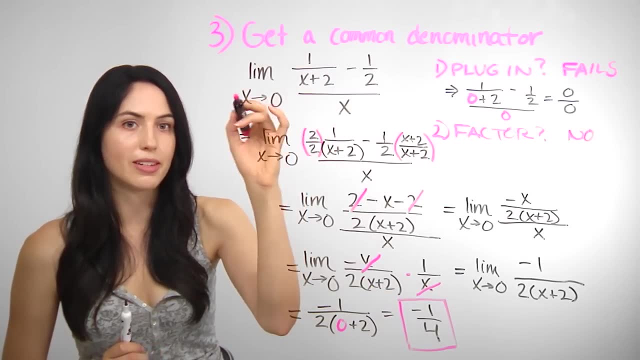 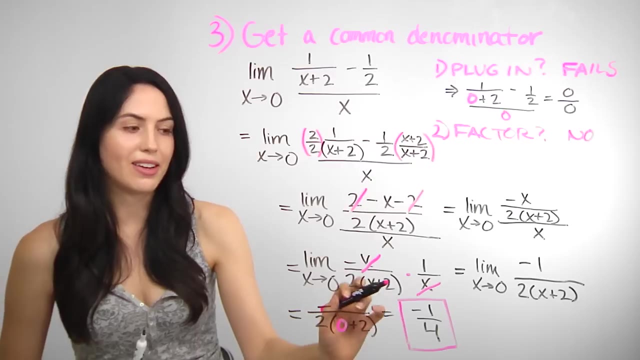 able to plug in 0 and get an actual number, an actual finite value: negative 1 fourth. So the limit of this expression, as x approaches 0, is negative 1 fourth. And yes, it's definitely okay to have a negative number as your limit. That just means that your function is approaching. 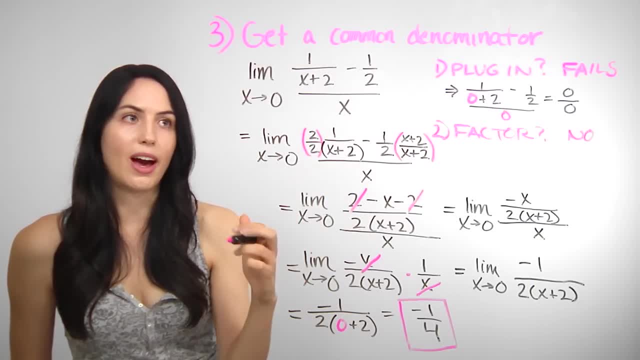 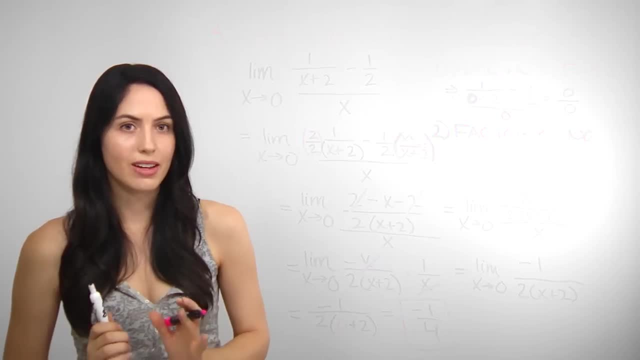 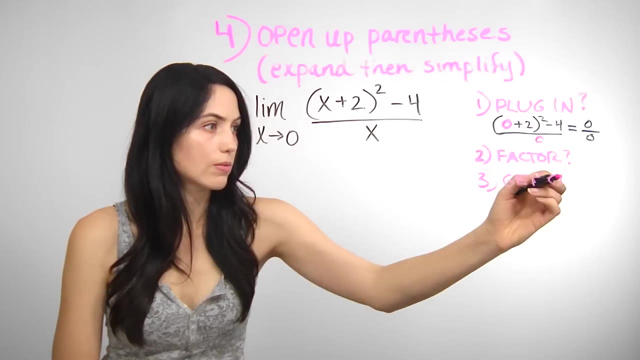 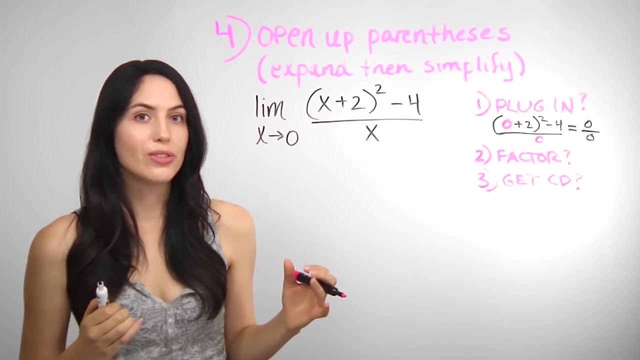 a negative number as a y value As x approaches 0, it's completely valid. So there's one more common method I want to show you, so let's take a look at that. Okay, here's another common type- Less common, but still useful. But first, definitely still. 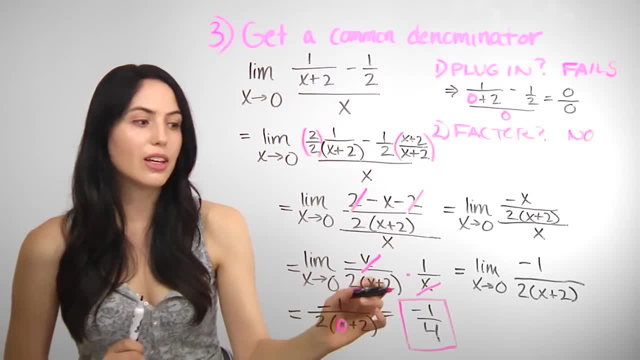 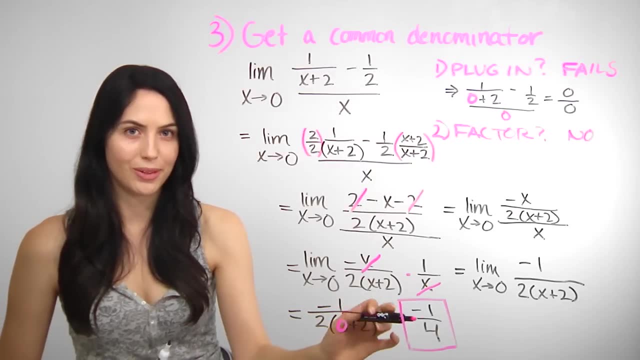 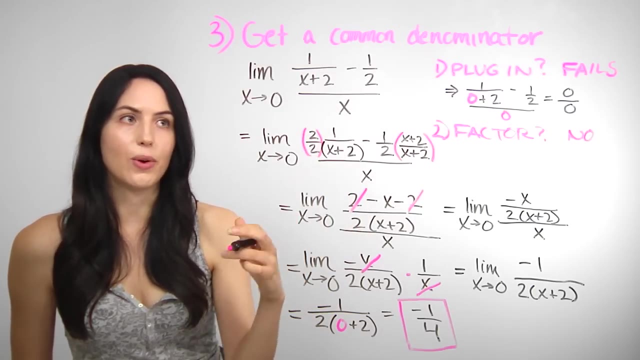 So the limit of this expression as x approaches 0 is negative 1. fourth, And yes, it's definitely okay to have a negative number as your limit. That just means that your function is approaching a negative number as a y value as x approaches. 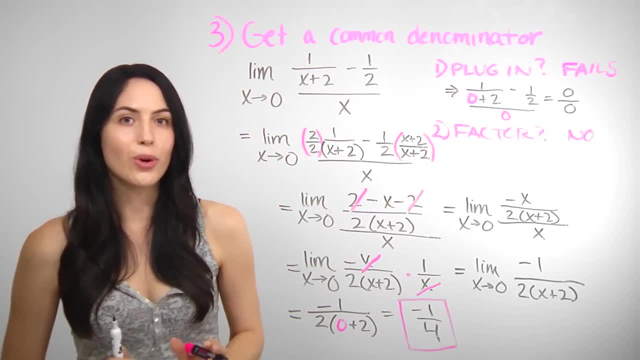 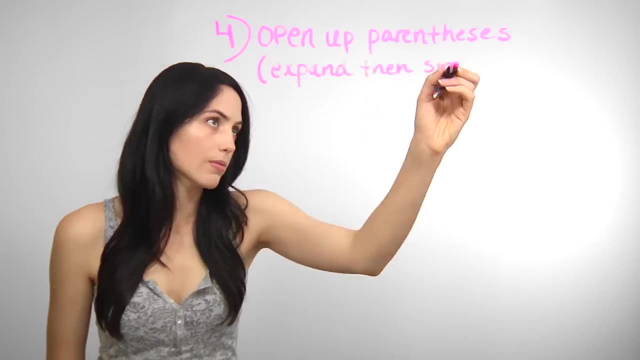 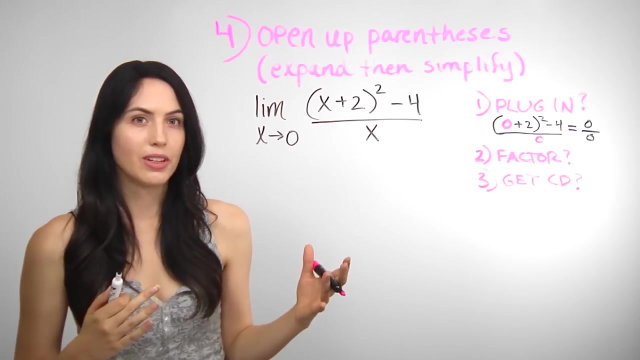 0. It's completely valid. So there's one more common method I want to show you, so let's take a look at that. Okay, here's another common type, less common but still useful. But first definitely still try your steps. 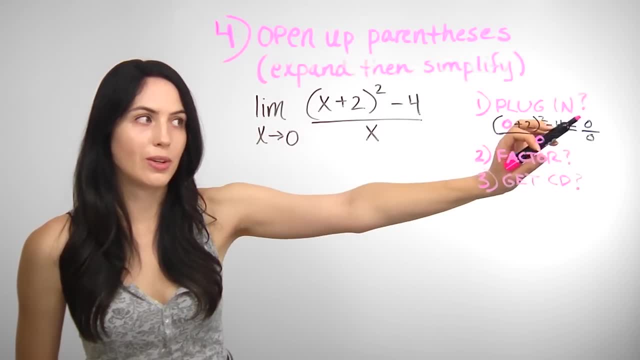 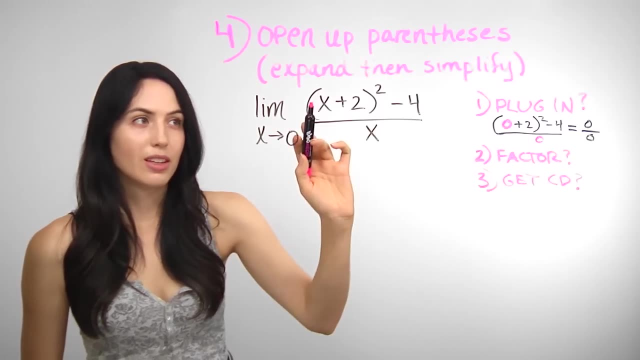 Try to plug in. When you do plug in 0, unfortunately you get 0 over 0, so you have to move on, try something else. So ask yourself if you can factor. There's really nothing to factor. there's nothing that's common to pull out here between. 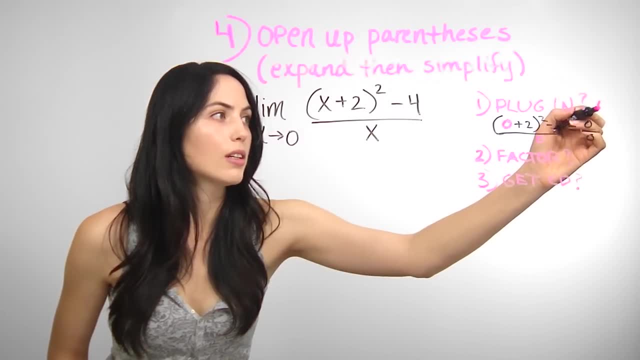 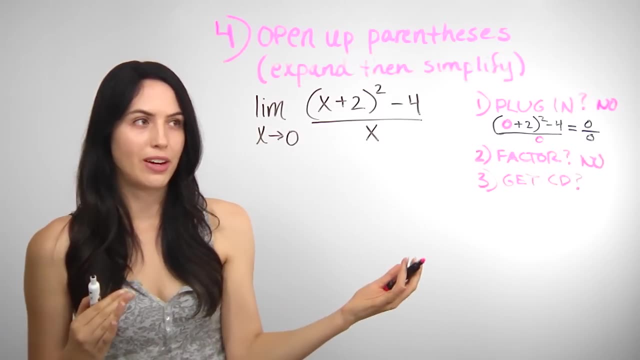 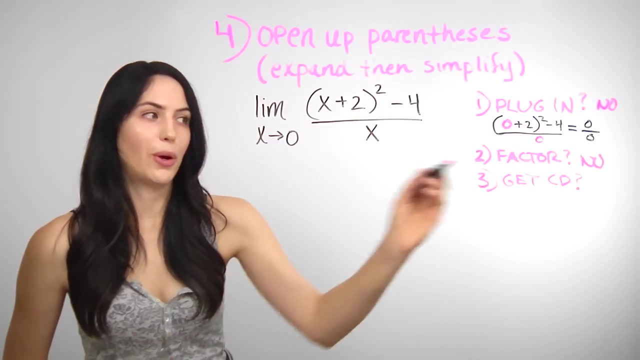 these terms. so no plug in no factor. no, then ask yourself, can I get a common denominator here in this expression? Well, no, there's really nothing to get a common denominator between. so no Then as a fourth approach. 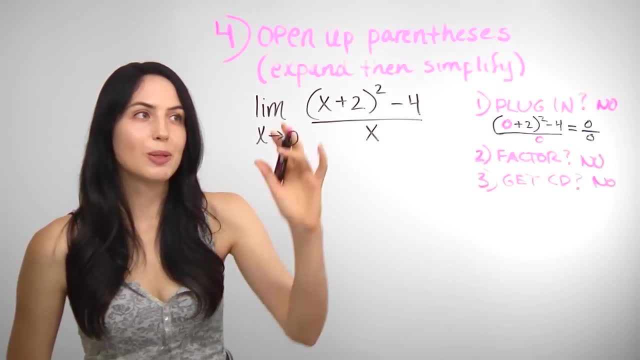 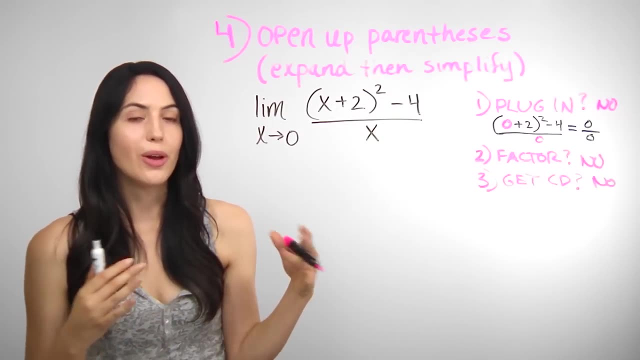 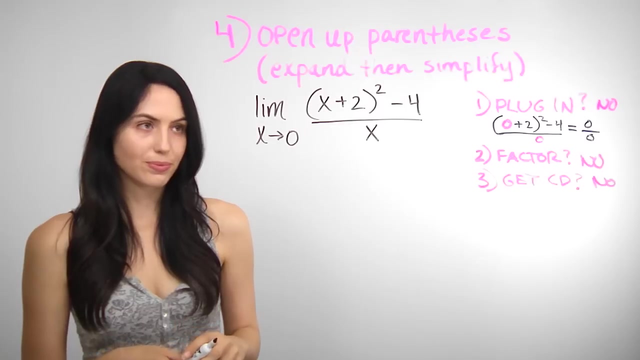 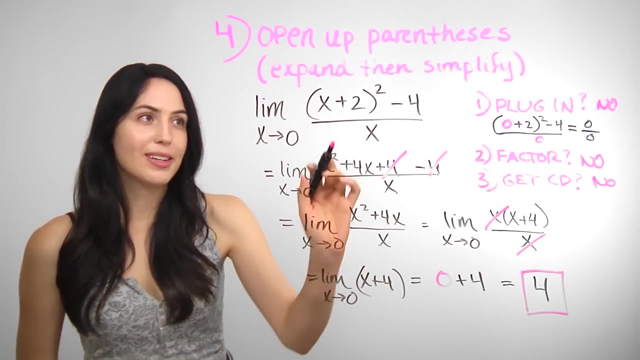 Okay, See if you can expand everything, multiply out, distribute, FOIL and then simplify so that hopefully something cancels and you'll be able to just plug in in the end and take and find a limit. Okay, take a look at this problem. so, basically, just by expanding, opening up these parentheses. 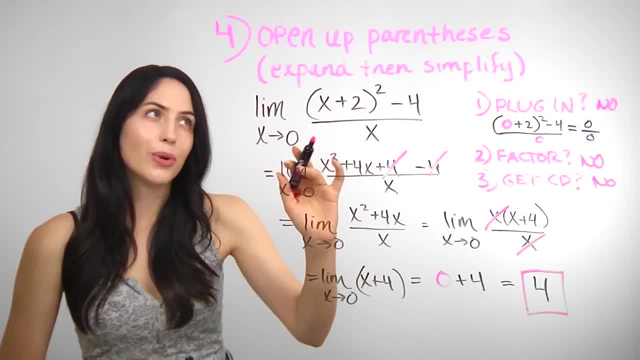 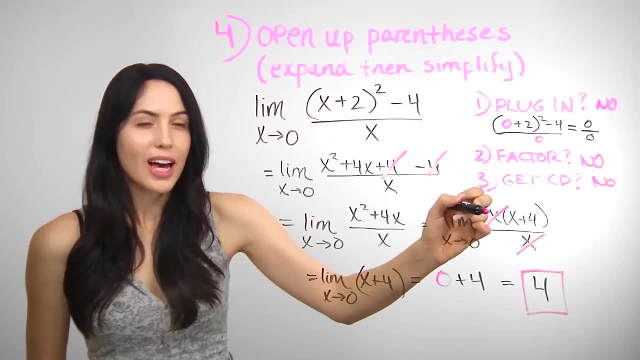 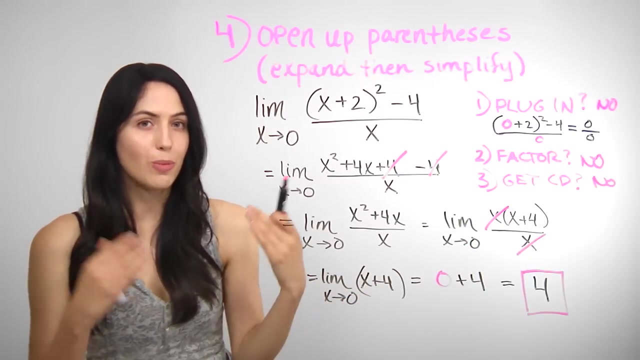 multiplying out, distributing, FOILing, we're able to simplify Terms cancelled. here that helped. and then later on we have to factor again. at this point pull out an x so that the x terms will cancel, so that more terms cancel and in the end 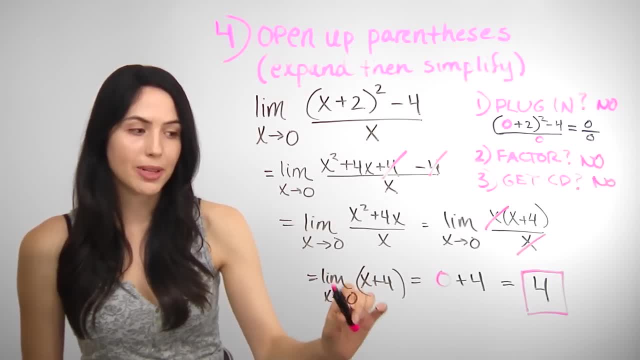 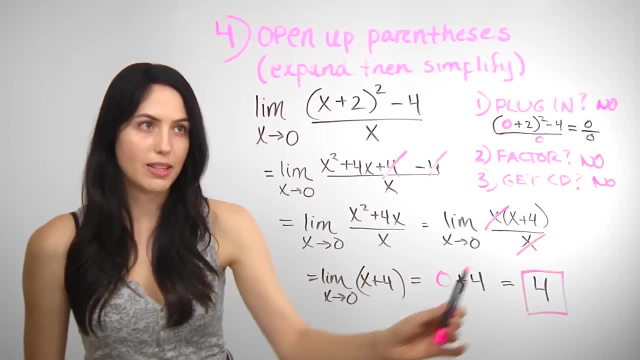 we're left with an expression that's simple enough for us to be able to plug in 0 and get a number, a finite value, For the last time. Okay, So that's the end of the limit. so the limit as x approaches 0 is 4.. 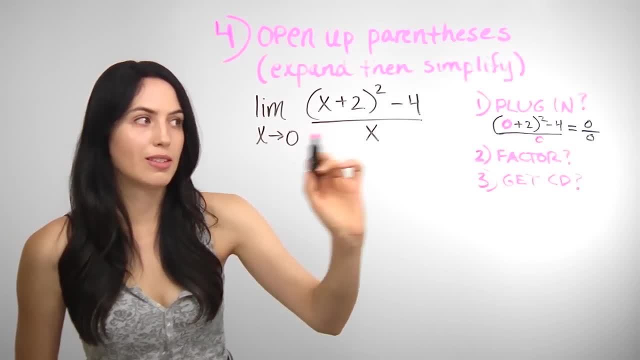 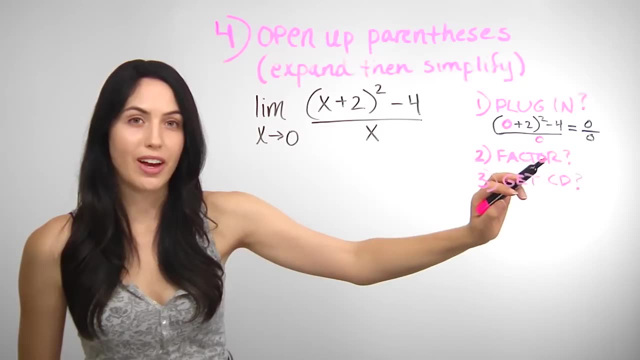 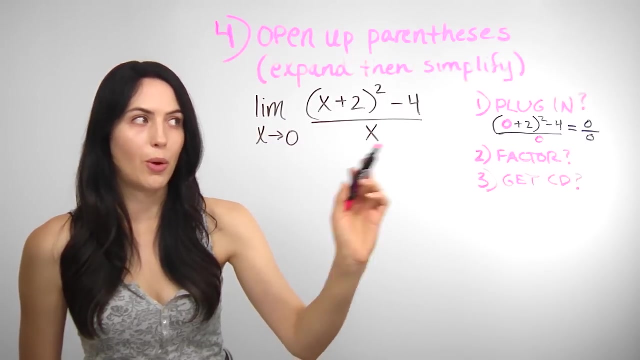 try your steps. Try to plug in. when you do plug in, 0. Unfortunately, you get 0 over 0, so you have to move on. Try something else. Ask yourself if you can factor. There's really nothing to factor. There is nothing that's common to pull out here between these terms. 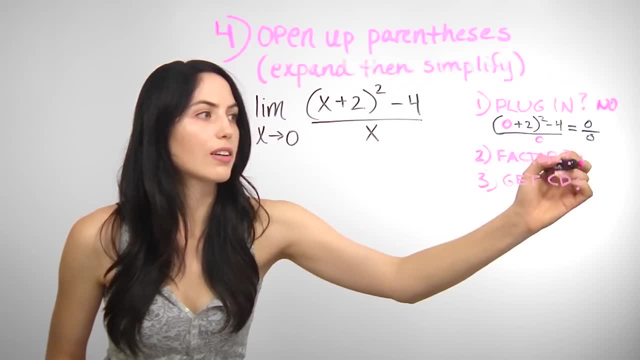 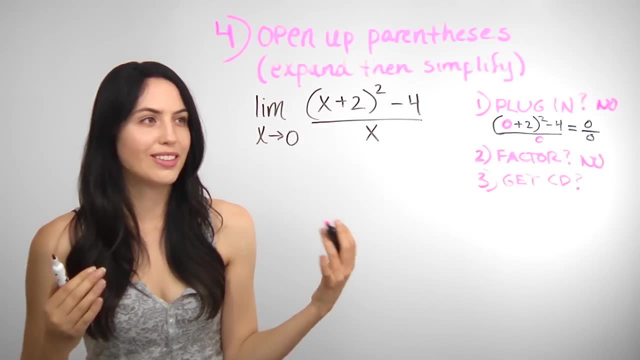 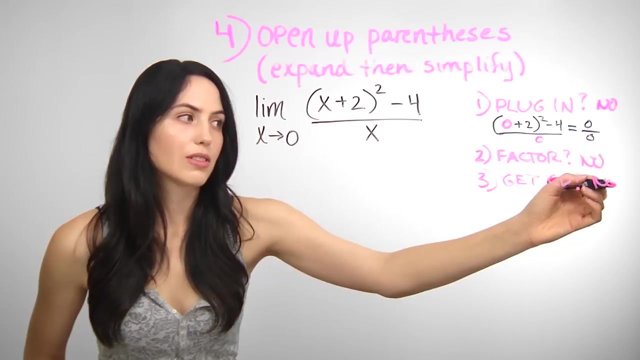 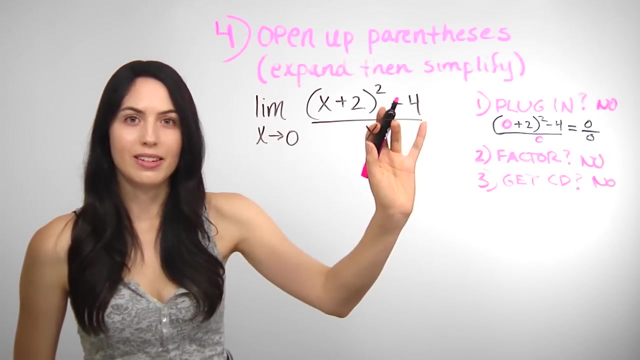 so no, Plug in, no Factor. no. Then ask yourself, can I get a common denominator here in this expression? Well, no, There's really nothing to get a common denominator between. so no. then, as a fourth approach, see if you can expand everything, multiply out. 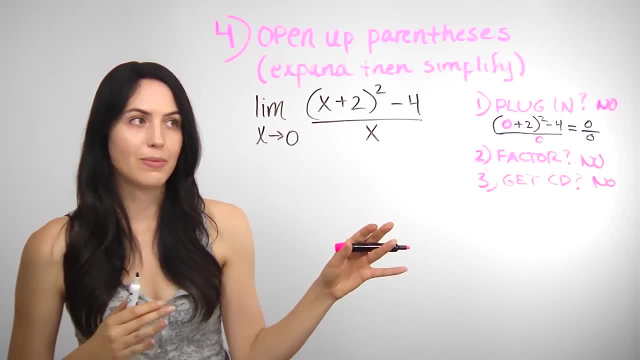 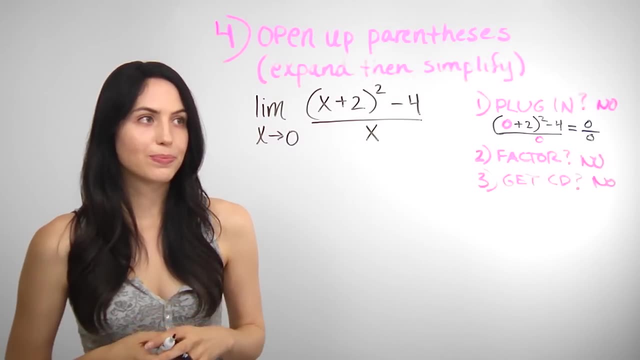 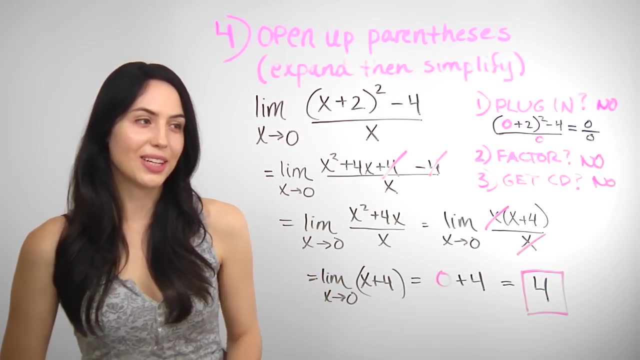 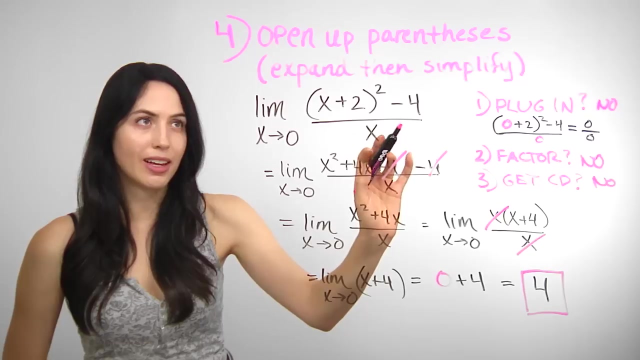 distribute foil and then simplify so that hopefully something cancels and you'll be able to just plug in in the end and take and find a limit. okay, take a look at this problem. so basically, just by expanding, opening up these parentheses, multiplying out, distributing foiling, we're able to simplify terms. 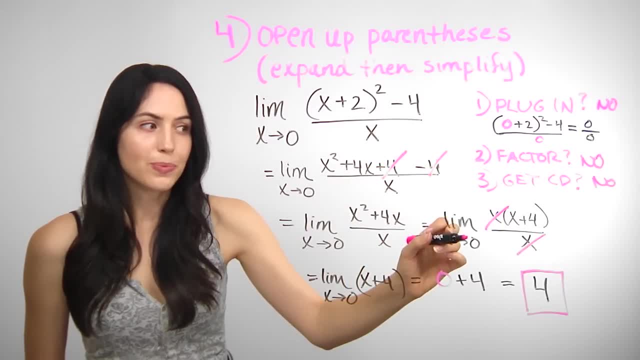 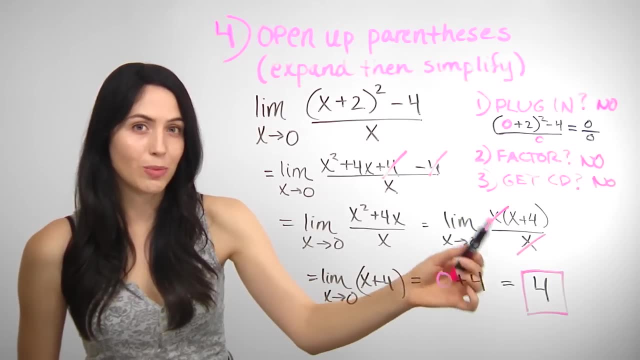 cancelled here. that helped, and then later on we have to factor again at this point, pull out an X so that the X terms will cancel, so that more terms cancel, and in the end we're left with an expression that's simple enough for us to do that. so that's the first step, and then the second step is to do the next step. 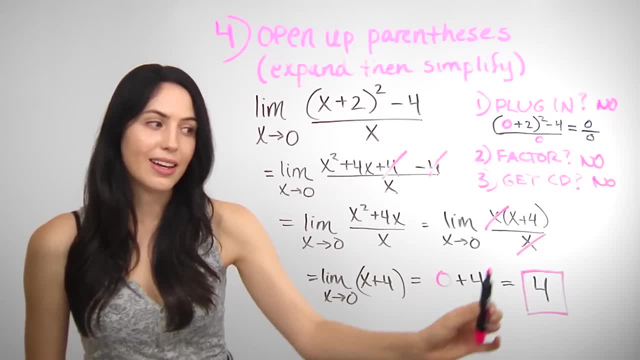 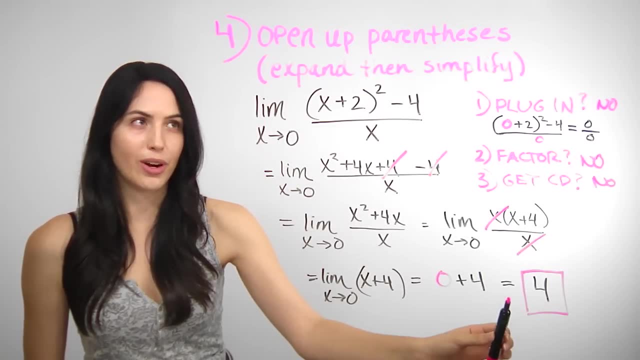 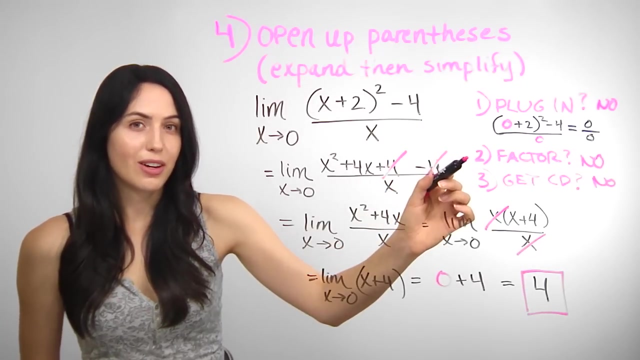 to be able to plug in zero and get a number of finite value for the limit, so the limits as X approaches zero is four. so just as a summary, remember the four most common steps for most common techniques approaches to try are: plugging in, factoring, trying to get a common denominator and expanding. 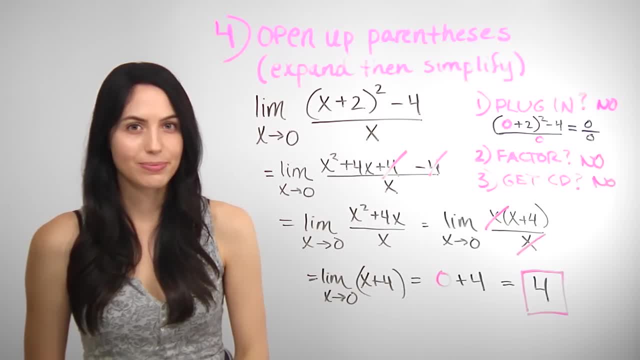 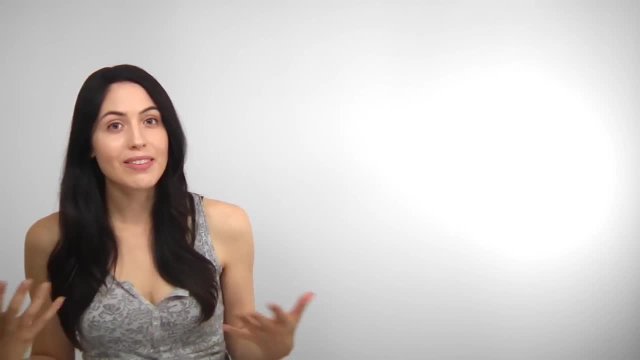 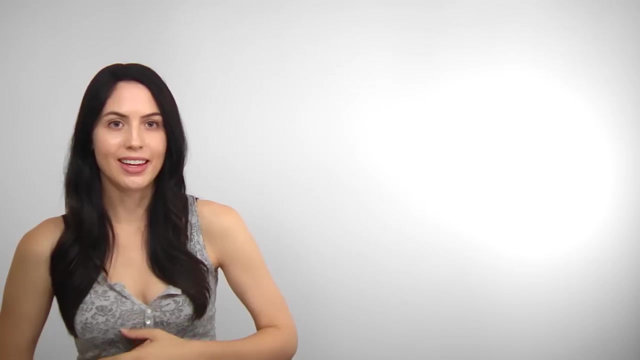 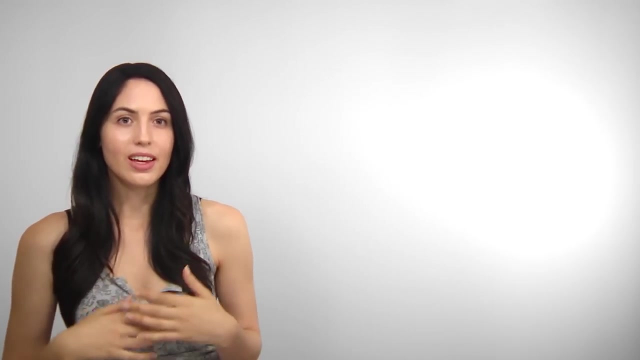 opening up parentheses and simplifying. okay. so here are some common things that tend to trip people up. sometimes people just give up too early. they'll plug in a number and they get zero in the bottom or zero over zero and they think they're done. that that's the limit, or that means the limit doesn't exist, not necessarily. 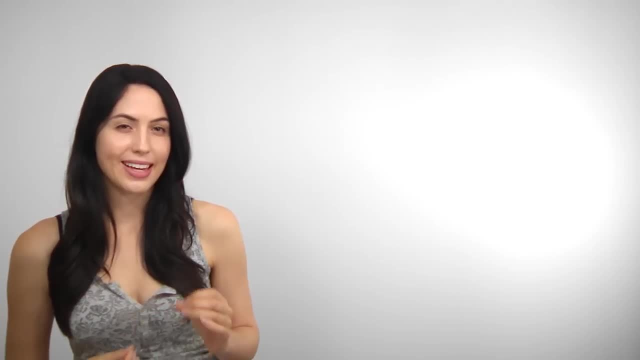 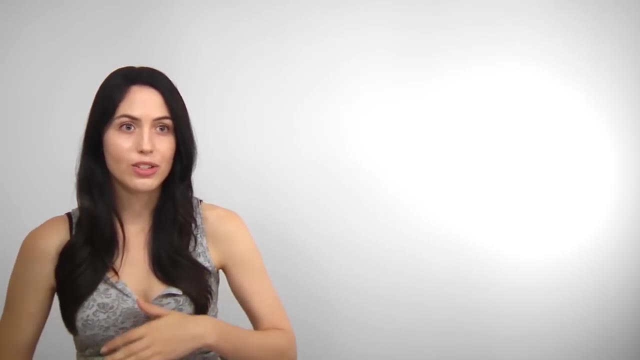 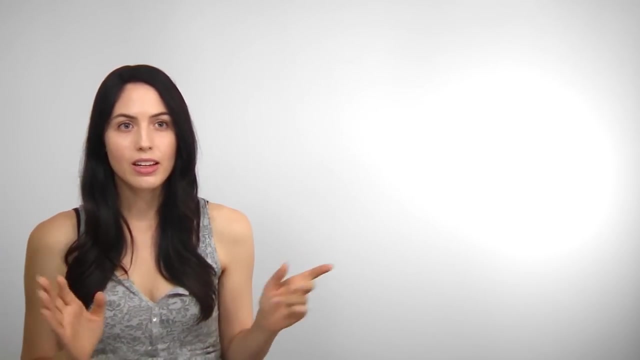 you have to try something else to try to get the limit number of the finite limit value. another thing that trips people up is that they just forget that they have these algebra techniques. don't forget, when you see an expression and it looks complicated, that you don't forget that you can factor, you can find. 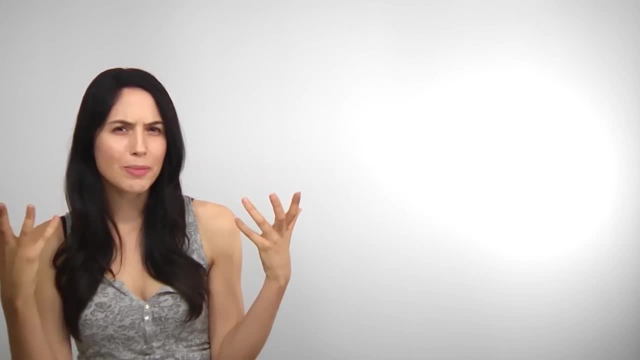 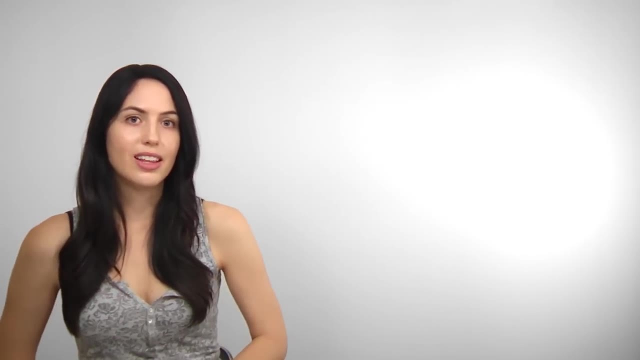 a common denominator. you can try to just expand, use what you know about algebra to try to make that expression simpler and probably in the end you'll be able to just plug in and get a number. and then one final thing, if you're, if you feel like you got off track. 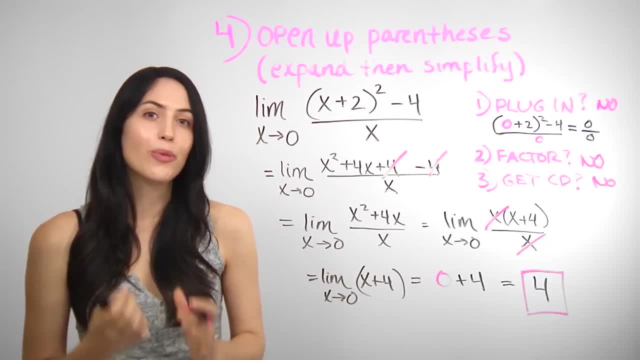 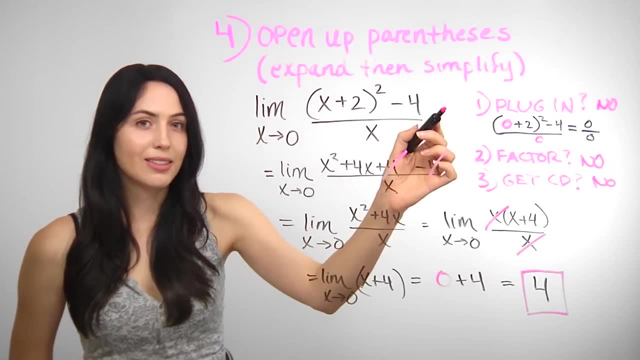 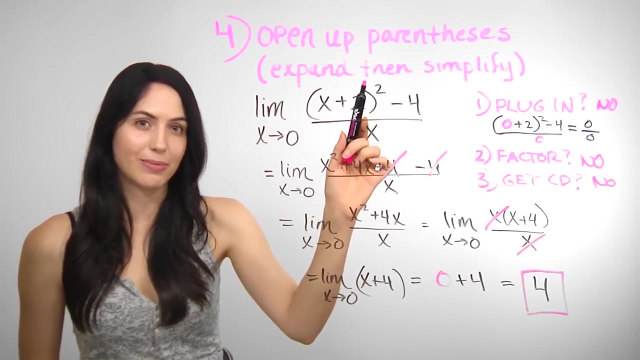 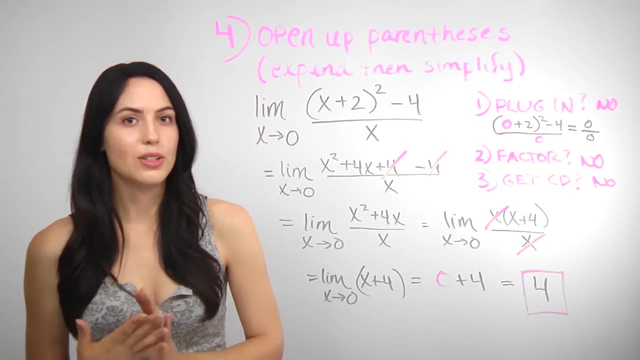 So, just as a summary, remember the four most common steps, four most common techniques. approaches to try are: plugging in, factoring, trying to get a common denominator and expanding, opening up parentheses and simplifying. Okay, so here are some common things that tend to happen. 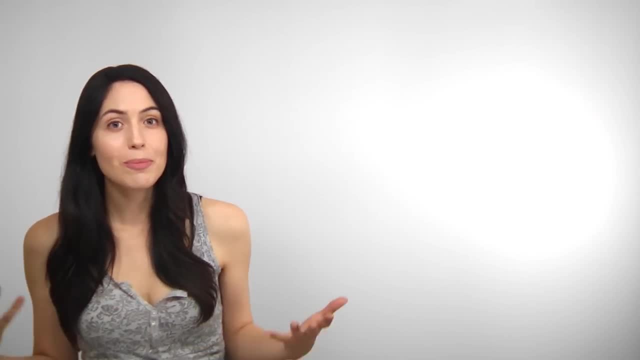 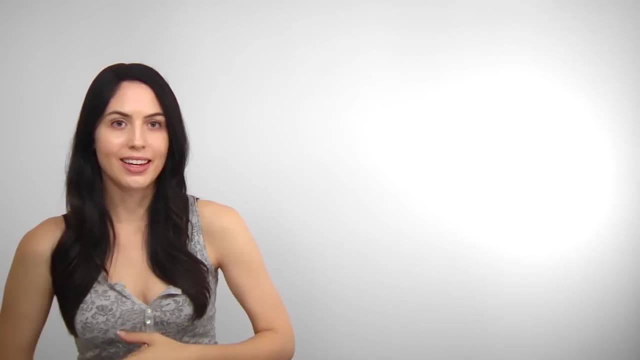 The first is to trip people up. Sometimes people just give up too early. They'll plug in a number and they get 0 in the bottom or 0 over 0, and they think they're done, that that's the limit, or that means the limit doesn't exist. 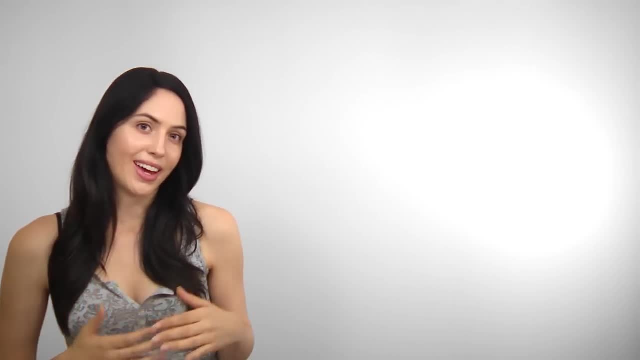 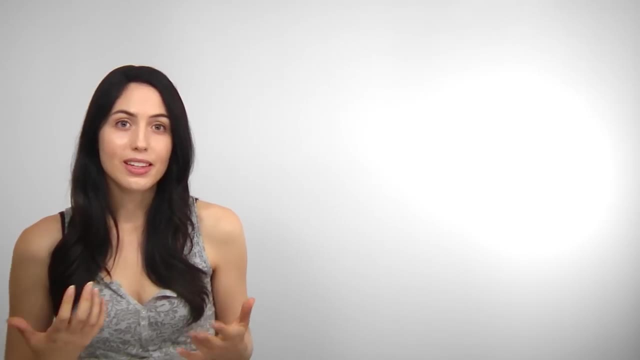 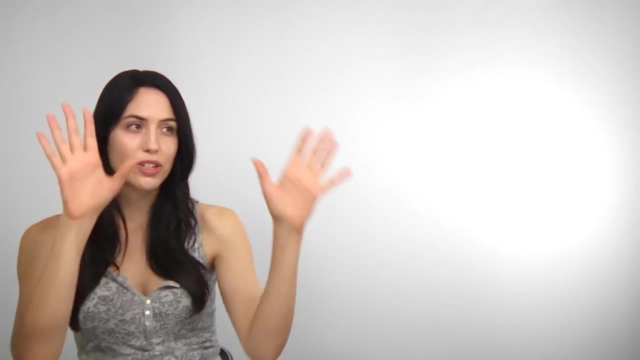 Not necessarily. You have to try something else to try to get the limit number, the finite limit value. Another thing that trips people up is that they just forget that they have these algebraic techniques. Don't forget when you see an expression and it looks complicated, don't forget that. 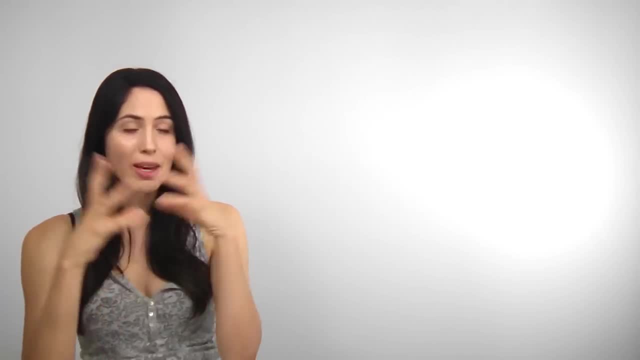 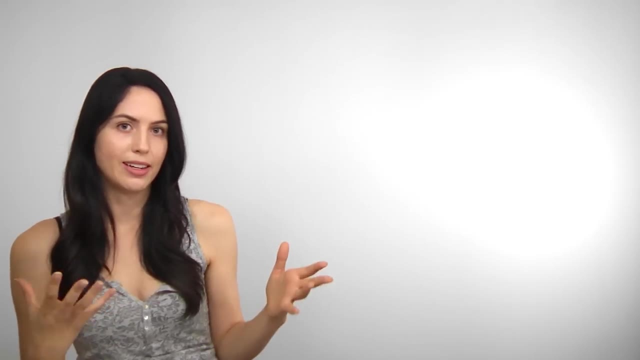 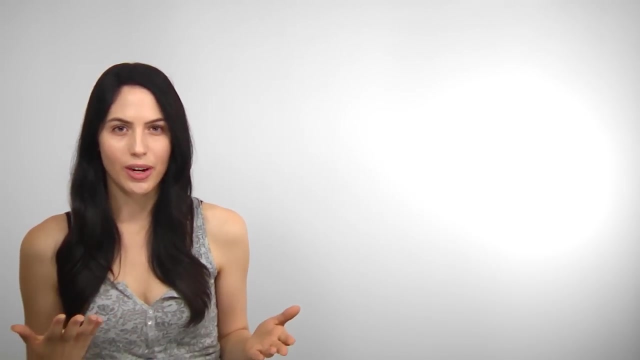 you can factor, you can find a common denominator, you can try to just expand, Use what you know about algebra to try to make that expression simpler and probably in the end you'll be able to just plug in and get a number. And then one final thing: if you feel like you got off track, try checking your work. 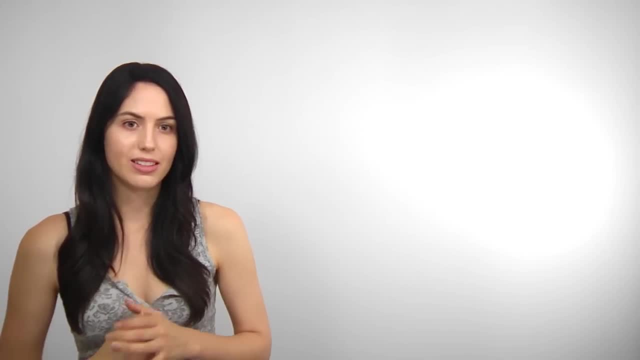 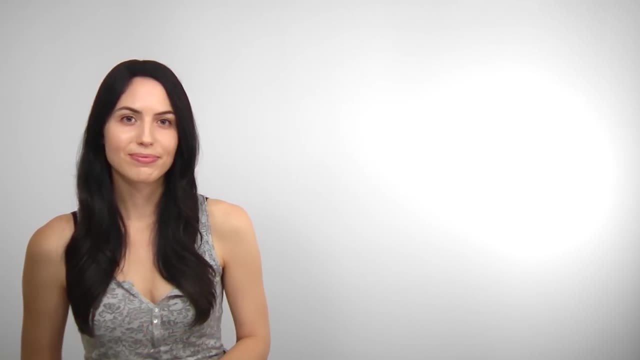 because it's so much algebra in some of these limit problems that there's so much nitty-gritty. it's really easy to make little mistakes, so it's worth taking a second look at your work. Okay, so those four approaches we just covered are the most common ways of finding a limit. 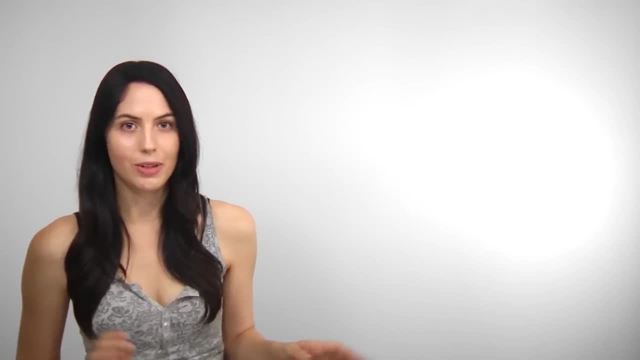 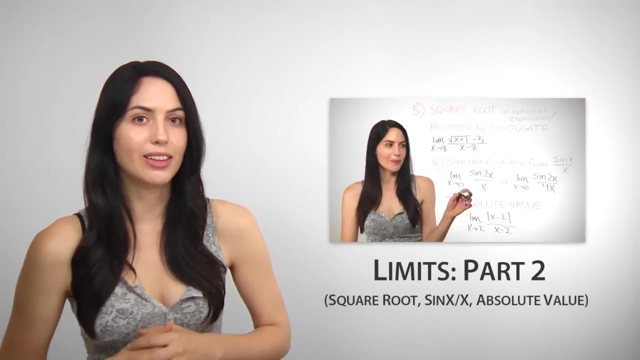 out of value. They probably cover 90% of those problems that you'll get, but there are about three exceptional types where you'll need special approaches to find the limit. so I made a separate video explaining those. So if you're looking for linear algebra, you're going to want to look at the first. 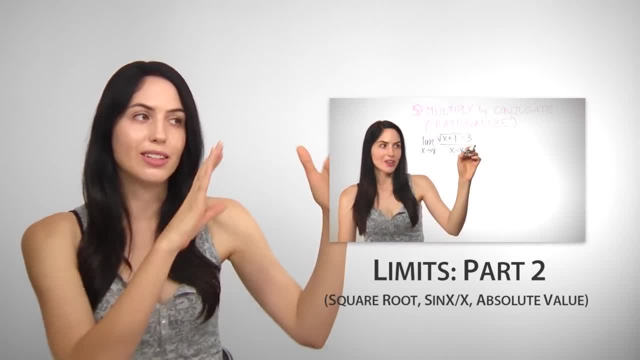 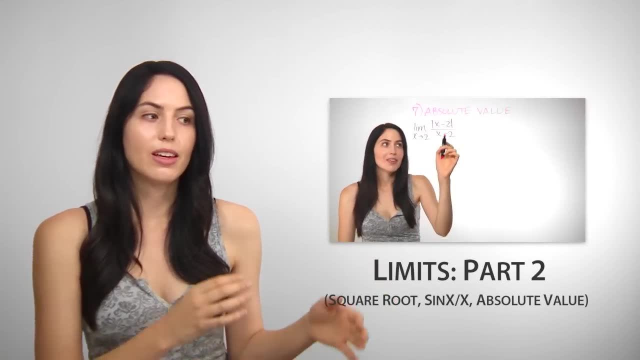 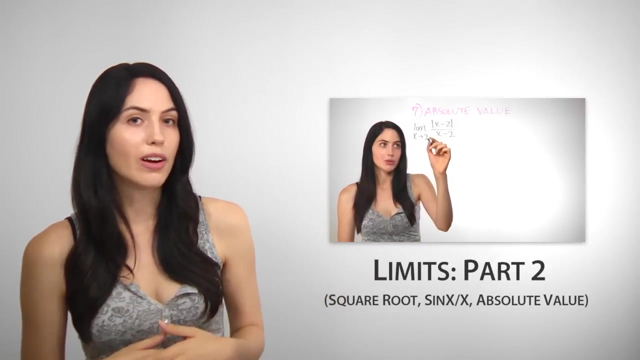 one which is the linear algebra of the equation. So, for example, you want to think of the equation of the formula. So let's say you have a formula that has a square root in the numerator of a fraction and you need to rationalize it by multiplying by a conjugate.